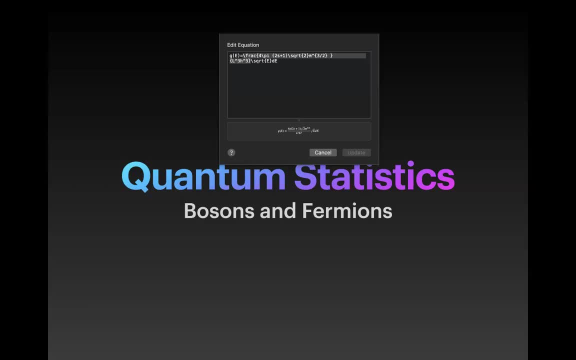 statistics about these different types of particles and what states they can be on, so namely bosons and fermions. so today we're going to start with looking at um, those quantum statistics. so first let's look at what's the limitation of classical statistics. um, so we talked about uh. 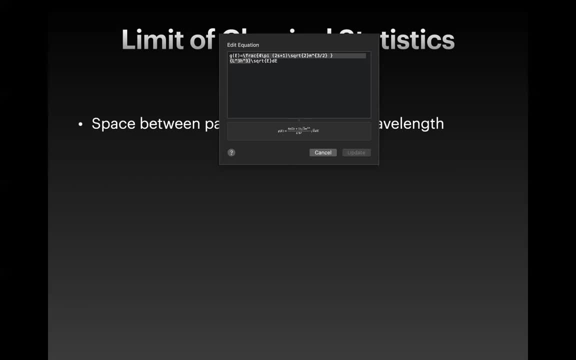 last Friday, um there's this very classic term that we call um 解 vị. if you look at the distance that we're talking about, right, so we can have a very long possible if that value is much less than one. what it means is most quantum states are unoccupied. 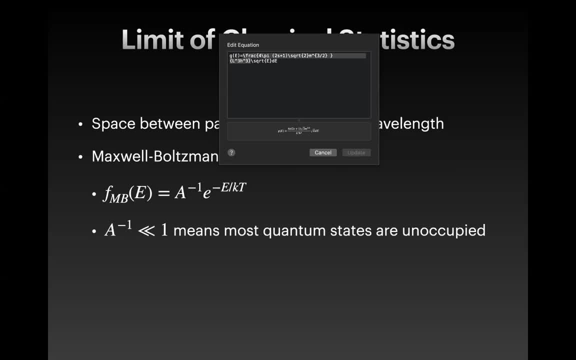 right. so if there, if so, we're not looking at interactions in the sense of a force between particles. the only way that these particles, um affect each other is if, like um there are, there, starts to be, you know, things start to fill up, right, so you might think of like um. 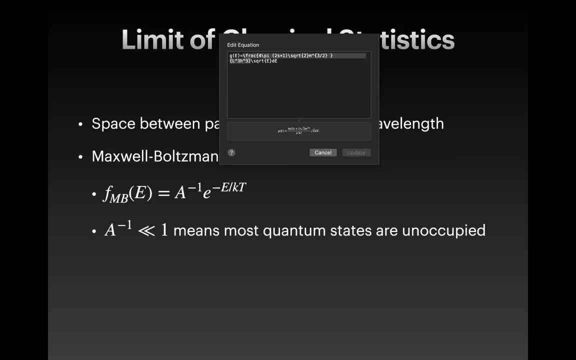 you know if you're in a large movie theater or um sports arena? um, you know, if you went there right now, right, you'd have your pick of whatever seat, right? because, because nobody's supposed to be there, right, and even as things start to fill up, you're not really necessarily going. 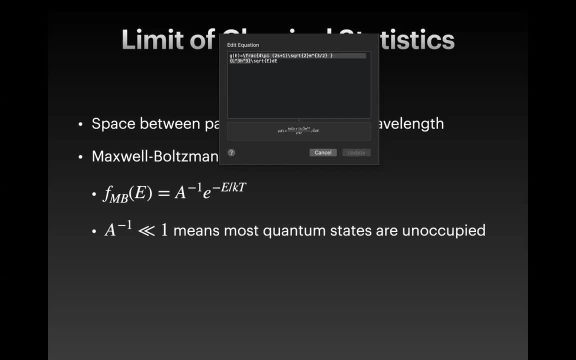 to interact with anybody. nobody's pushing you right, but, um, at a certain point you can't pick just whatever seat you want, right, because they're full right, um. but if the occupation number is really small, then you basically get whatever seat you want, but as it starts to fill up, then there's only certain ones left over. so that's kind of what we're. 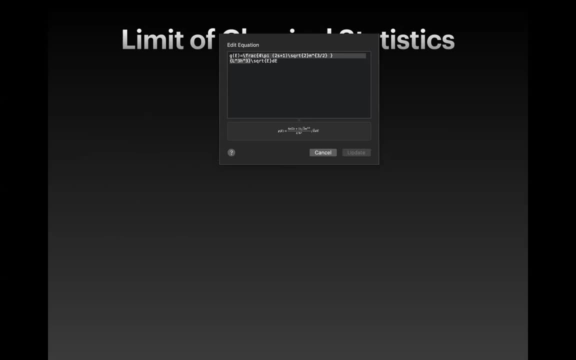 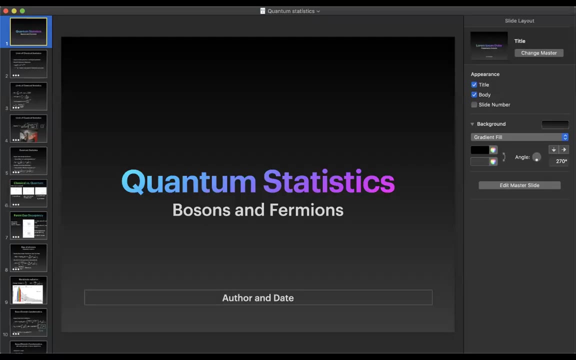 looking at here. hey, dr bartz. yes, uh, we have a, at least i do. i have like an edit equation box in the middle of my screen. yeah, same here. huh, i don't know if it's from: oh, am i, maybe i'm? i don't know. yeah, it's just blocking the uh. 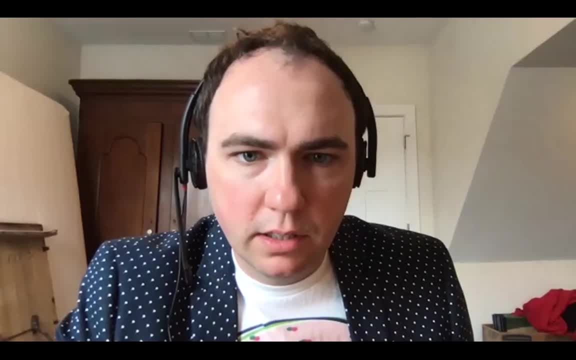 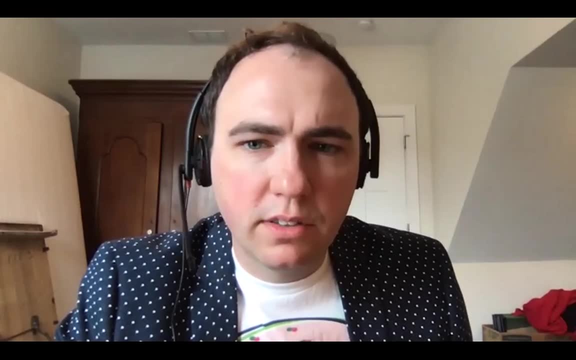 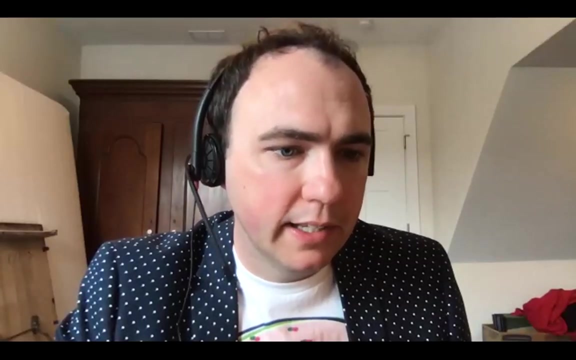 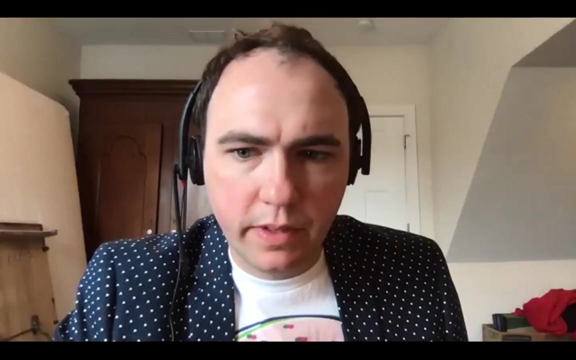 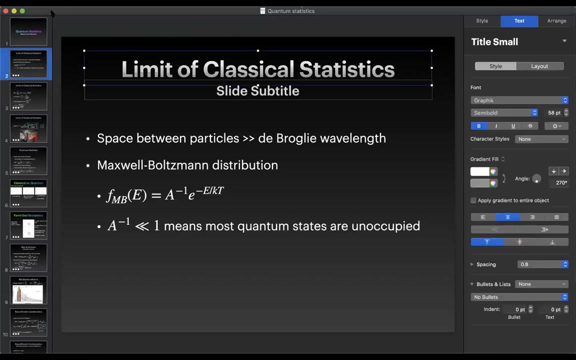 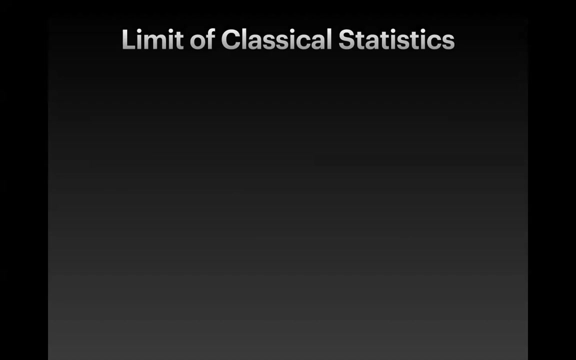 let me um, okay, let me. aha, that's my other window. okay, i'll close my other slideshows. thank you, yep, okay, so let me go back and share this again, that's okay. so let's go back to our first question. if you need information, um, you can. um, you can direct it to the city, or uh. 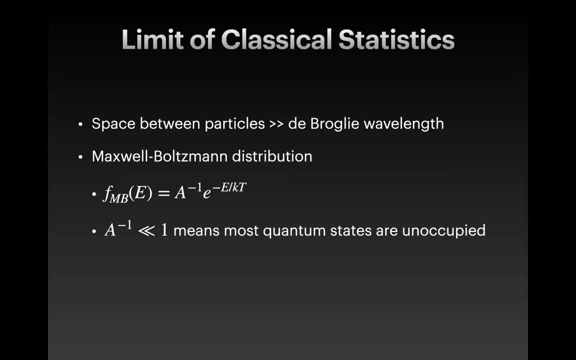 um, now, if you need information, um, um, i'm going to have to go back and check um, so, like i said, you can direct your question to me, um, and then i'm going to go ahead and, um, send it back to me and then, um, the other thing, i just wanted to make sure that. 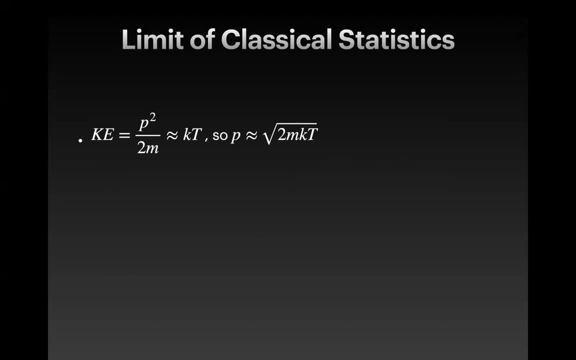 i make sure that everyone's going to be able to see it, right, uh? and so i did that right. so i'm going to state this to you non-relativistic. so kinetic energy is p squared over 2m, which is approximately Boltzmann constant times temperature. Now we found that, you know, the average is one-half kT. 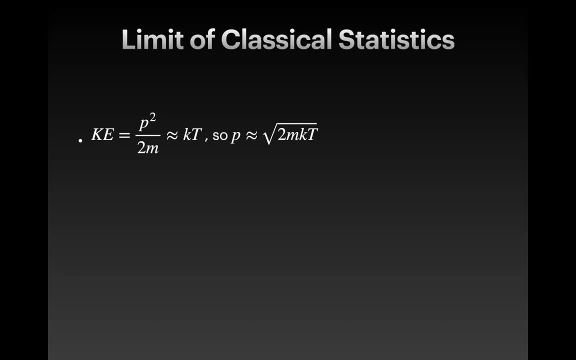 or sorry. the most common energy was one-half kT and the average energy was three-halves kT. but if we're just kind of rounding and saying what's you know, what's the scale of the energy, we can just use kT and not worry about that numerical factor. So momentum is going to be. 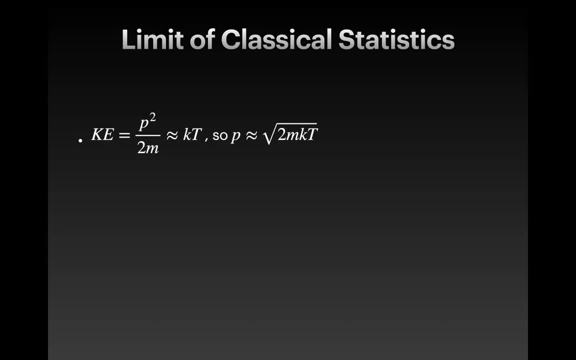 square root, 2 times the mass of the particle, times kT. So then we have the de Broglie wavelength. right is Planck's constant divided by the momentum. so we can write that in terms of the temperature using that calculation and the particle separation is well. if we take the 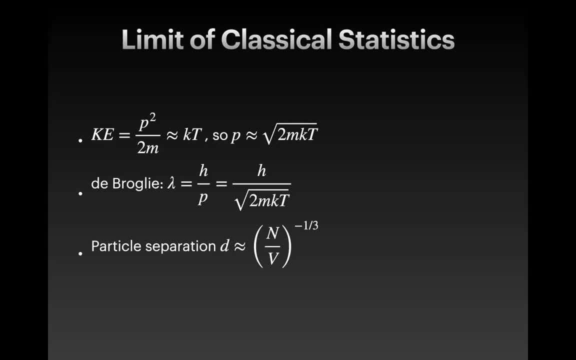 density of particles. right, the number of particles divided by the volume, that's going to be one over distance cubed. so if we take that to the minus one-third, that'll give us a distance, a separation distance. So the ratio of lambda divided by the particle separation is going to: 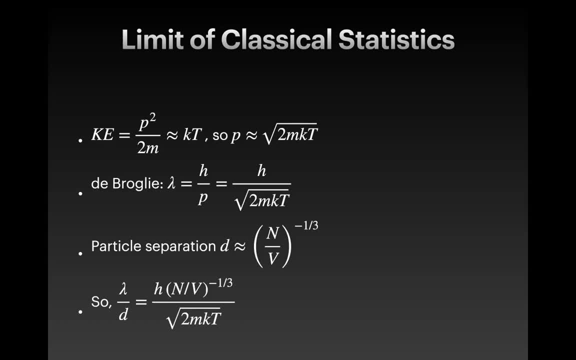 be given by this expression. right, so we just take the ratio of those two things. Okay, so we have that. Now recall this thing that I never actually wrote down, ultimate jerk move of a professor, but we had set up how we solved for this normalization. 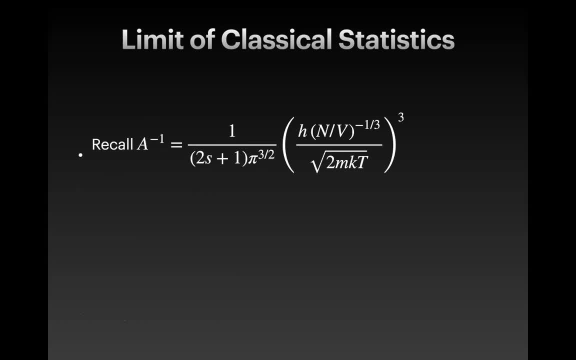 right, and it was by integrating the number density from energy equals zero to energy equals infinity, and then, okay, you know, setting that equal to the total number, right? so if we do that and rearrange it a little bit, I've put it in this way so that that part in the parentheses there is cubed. Okay, now let's. 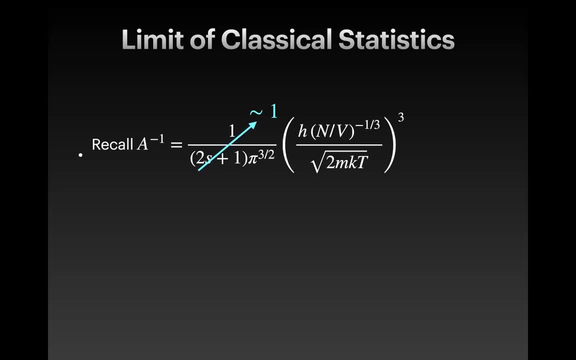 look at the part in front: It's order one, right, I mean it's not one, you know it's something over pi-ish, but order one, meaning it's not 10, it's not 0.1, you know it's not going to make a big. 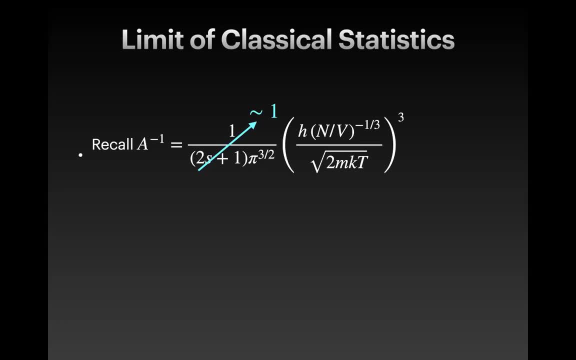 difference. So if we're just doing order of magnitude, what we need to look at is what's in the box, and hopefully you can see that that is, and if you can't, you know you can, you should be able to. 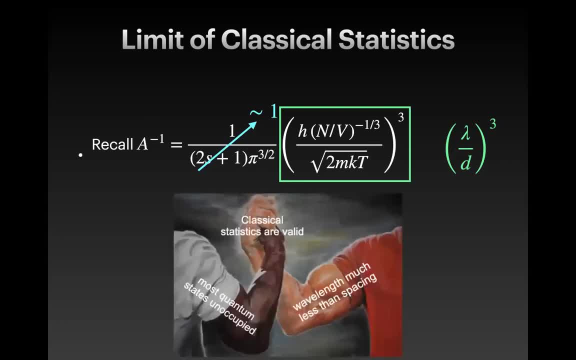 move the videos around, that is equal to lambda over the particle distance, right? So you know, had to put this in meme form, right? So saying that most quantum states are unoccupied and saying that the wavelength, the de Broglie wavelength, is much less than the particle spacing, is really two ways of saying. 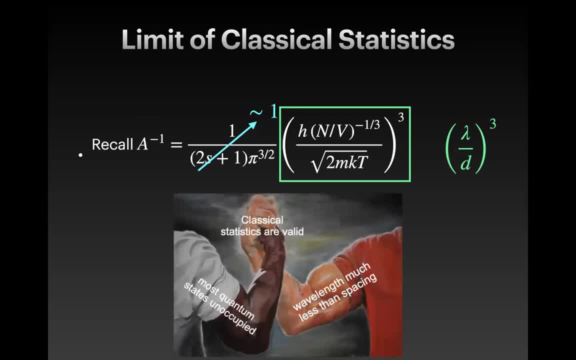 the same thing. So that was the point of saying this. right So that what we said was valid because of the meaning of this or the quantum meaning of this normalization. right, So classical statistics are valid. as long as that is the case, all right. So once that is no longer, 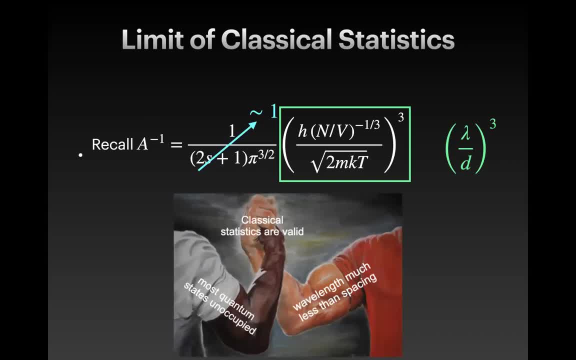 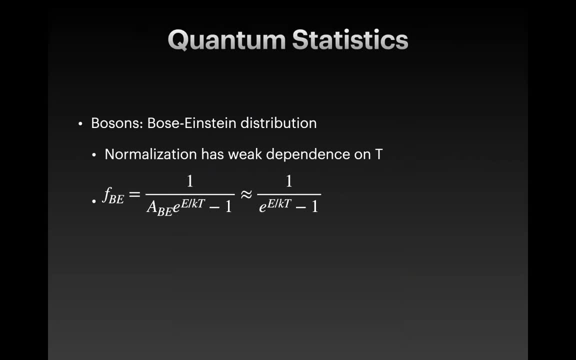 the case, then we have to do quantum statistics, and when we do quantum statistics we have to worry about what type of particles we have. Okay, So we got two types of particles, main types of quantum particles. We either have bosons, 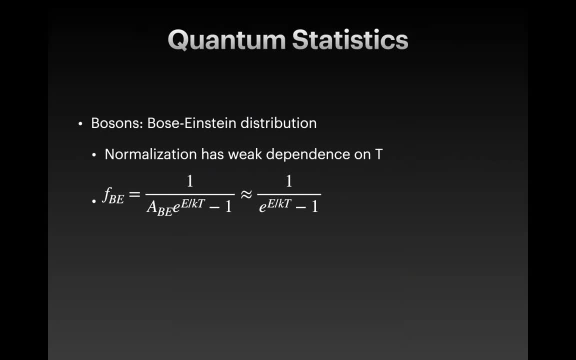 which follow the Bose-Einstein distribution. So we write this distribution right. So this is the probability of a particular energy state energy level being occupied. It's one over. okay, there's some normalization: a for Bose-Einstein, e to the energy over kt, and then 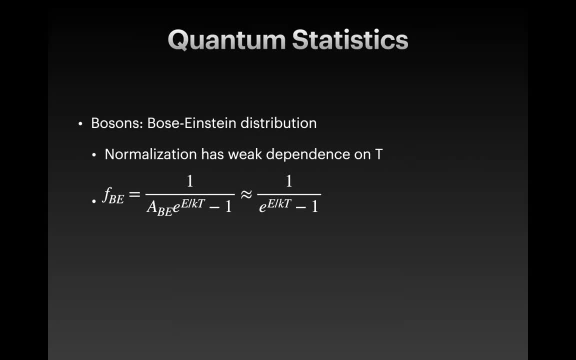 minus one. So for the most part for bosons the math actually gets hard if you try and do everything perfectly. but we're looking at big ideas here. So for bosons then that normalization factor doesn't really depend on temperature much. So we can basically set it to one, and so we get. 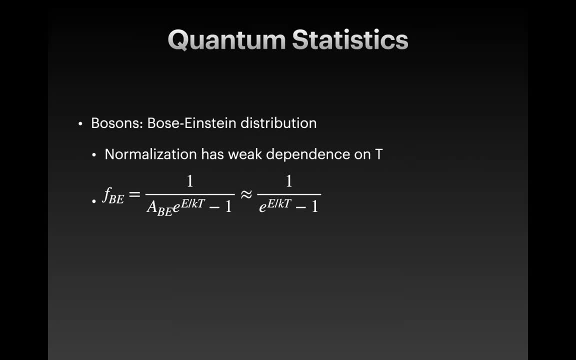 this simplification there. Now, if you, yeah, if you look at that denominator there, all right, we have e to the energy right normalized by kt minus one. So if we think about the limit where the energy is really high, wait. 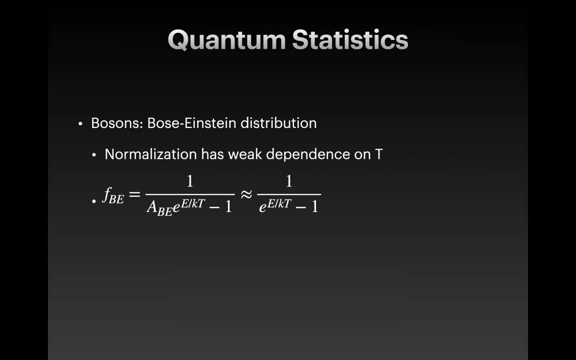 sorry, this is something that helps to, helps me to write, to say it, If the energy, so if the temperature gets large- no, forget what I, let's forget what I was going for there- What we should find is that in the high temperature limit- yeah, this would be the same. 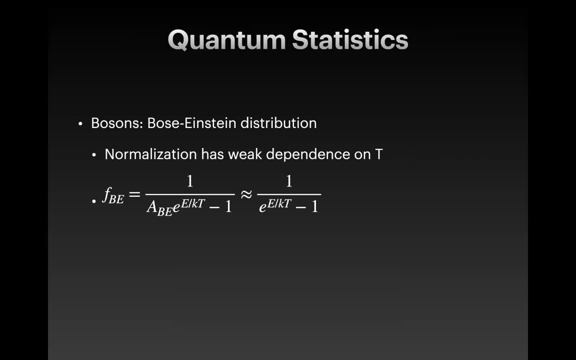 as the, as the Boltzmann Boltzmann distribution, right And in the low temperature. then we actually have to do quantum statistics. Our other option for type of particles is fermions. So they follow what's called the Fermi Dirac distribution, Now fermions. their key feature is that they obey the Pauli exclusion. 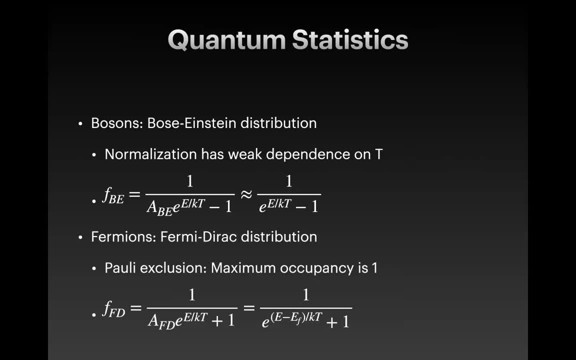 principle, right? So that means that you can't have two fermions that are in exactly the same state. In other words, the maximum value of this distribution function is going to be one, right? So it ranges between one and zero. Now it looks quite similar if you just write it. 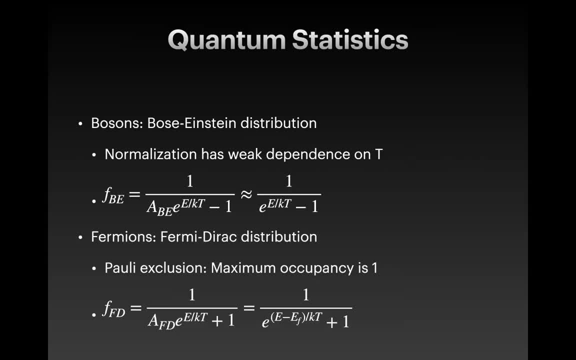 to the Bose-Einstein distribution if you just write it with the normalization there, but there's a plus one instead of a minus one. But the other main difference is that the normalization has a strong dependence on temperature for fermions. Right, So we can write that normalization as e to the negative e sub f, which is the. 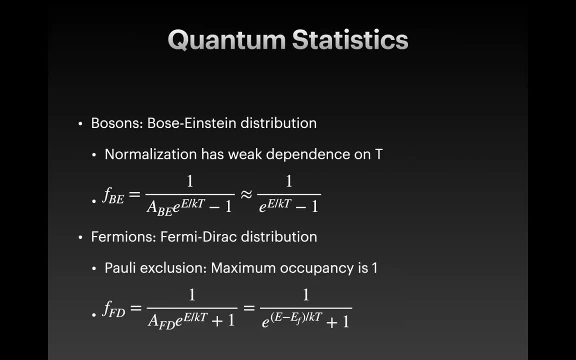 Fermi energy, which, you might recall, we talked about when we were doing the energy levels of neutrons and protons within a nucleus, right? So that's the Fermi energy that becomes important. Okay, so we got the expressions, but it's much easier to kind of see what's going on here if we 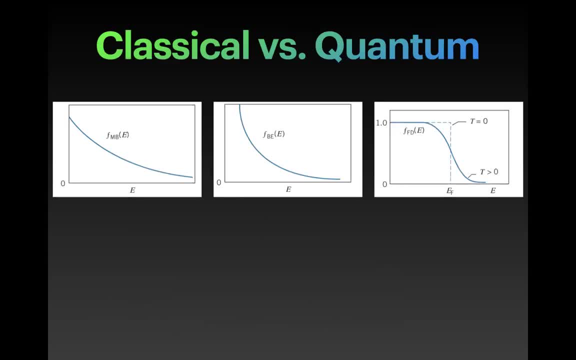 look at the plots: right So classical versus quantum. So on the left we have the Maxwell-Boltzmann distribution, In the middle we have Bose-Einstein and on the right we have the Fermi-Dirac distribution. 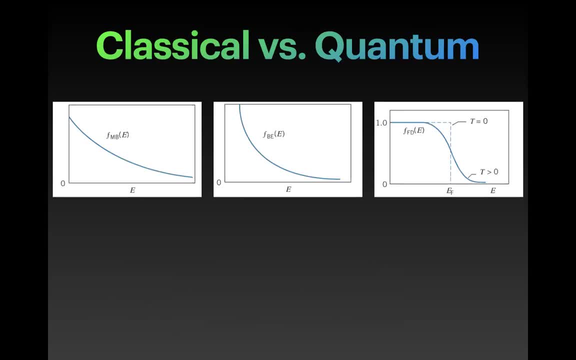 right. So the Boltzmann distribution is just a decaying exponential as energy goes up. Now this is at a fixed temperature, right? So at a certain temperature, what is the probability of having a certain energy? So the Maxwell-Boltzmann starts at some value and constant and decays to. 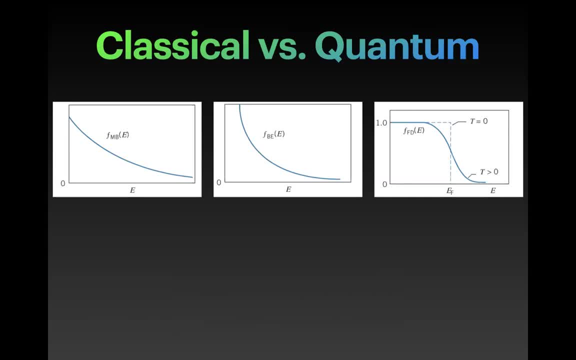 zero. The Bose-Einstein actually blows up to infinity at energy equals zero, And then the Fermi-Dirac distribution. so there's two plots there, right? So the dotted one is what happens at temperature equals zero. So at temperature equals zero, it's just going to be a step function. 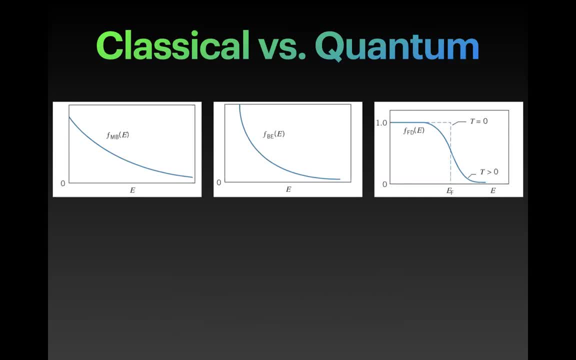 right, It's equal to one exactly up until the Fermi energy, and then it drops to zero. So all states below the Fermi energy would be occupied and then all states above the Fermi energy would be empty. Once you start raising the temperature, you get a more gradual transition. 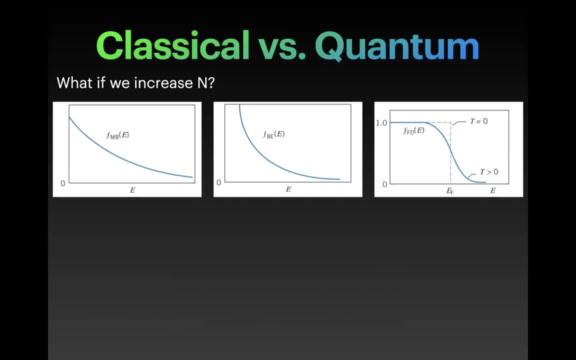 We'll look at that a bit more closely on the next slide. But now this is for a given number of particles. So what would happen if we increased — you know, if we added more particles to our system? Well, for the Maxwell-Boltzmann distribution, that's just going to shift the curve up. 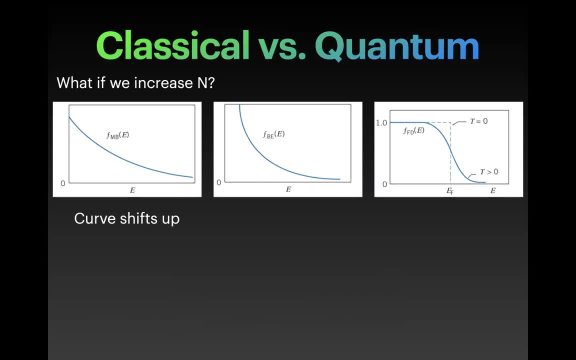 right. So we just have that normalization constant. You know, if we double the number of particles, we double that a inverse — that normalization constant, And so the whole curve would shift up and it would have twice as much area underneath it. The Fermi-Dirac distribution can't shift up. 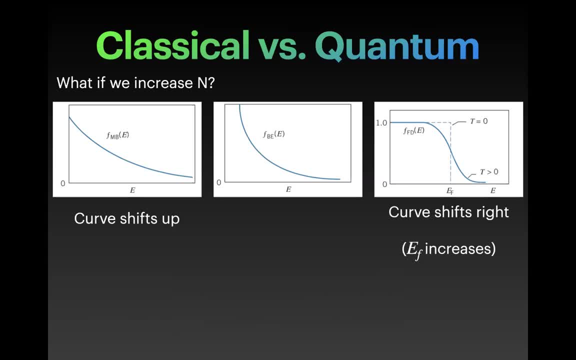 right, because it has a maximum value of one. So what happens is the curve actually shifts to the right, So the Fermi energy is going to increase, right? So as you, as you add more particles, the Fermi energy increases, And so that just means it's like: well, we, we kind of drew this picture. 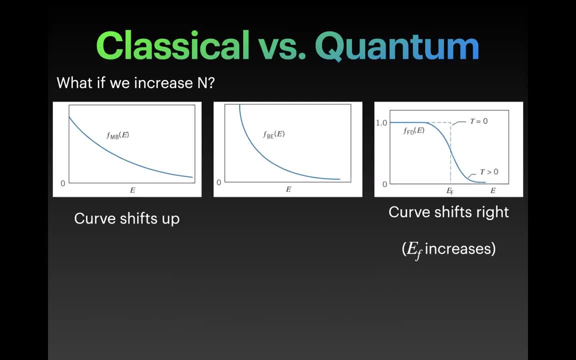 as we were putting particles in the nucleus right, You have these energy levels and if you want to add another one, it has to go into the higher, higher energy level. right, because everything up to here is full And then above that you can put, you know there's empty energy levels. 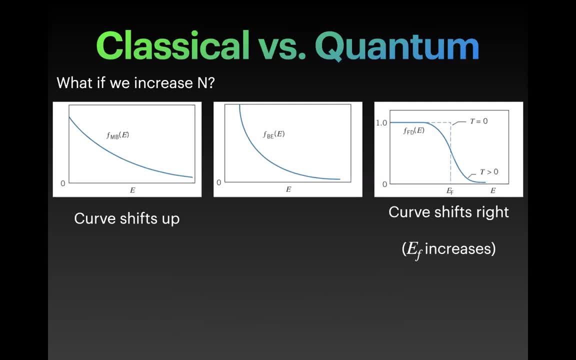 so you put another particle in there. Well, if you put another particle in there, the energy below which all states are filled is now above that. Okay, so that's that's how more particles get added With the Bose-Einstein condi or, sorry, with the Bose-Einstein statistics. I. 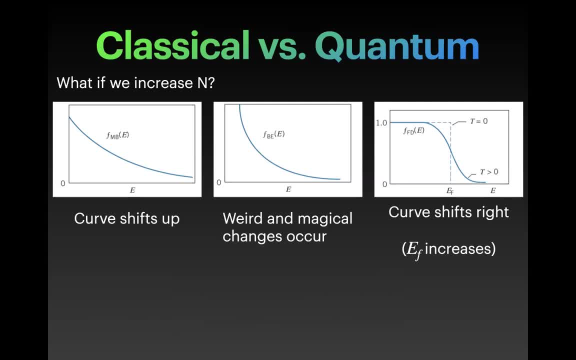 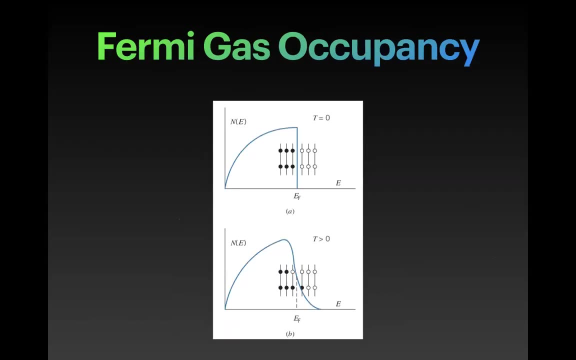 slip of the tongue, kind of gave away what what I'm going to go for. But weird and magical changes occur if you start to add more particles above a certain threshold value. So we will be looking more deeply into bosons today. Okay. so just kind of a clearer illustration of the Fermi gas Now. 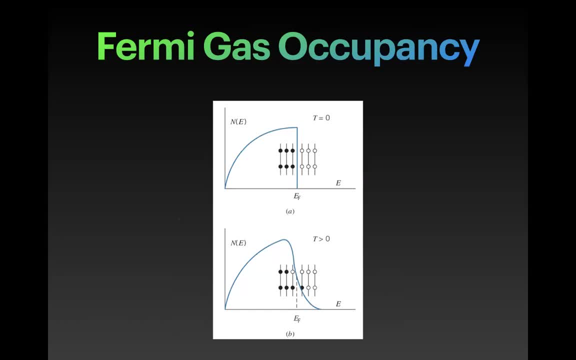 remember those plots I was showing before, were the, the distribution function, right? So that's just the- the probability of an energy being filled, but it didn't take into account the degeneracy or the- the number of different ways to have that. So if you multiply by the density, 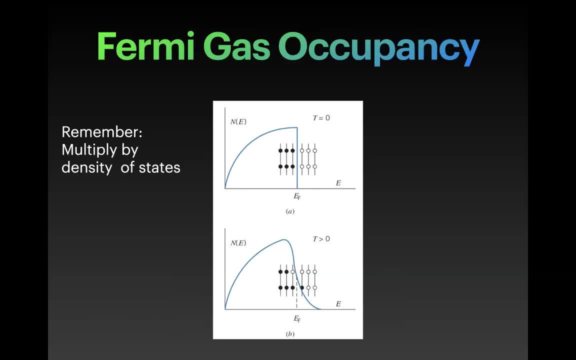 of states, which starts at zero and goes as the square root of energy. again, I'm mirrored, so I guess I should go this way. square root of it goes increases, with the square root of energy. for non-relativistic particles that means that basically you don't have any at energy equals. 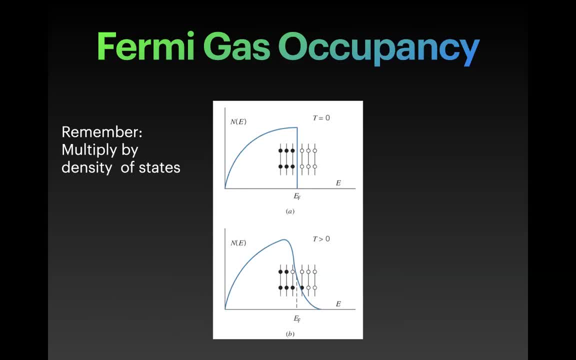 zero, Even though the probability is is one. it's just there's not a lot of ways to have zero energy for fermions or for any, you know, for non-relativistic particles, And then that's going to increase. but then when you're multiplying by zero, you know it still drops off instantly. 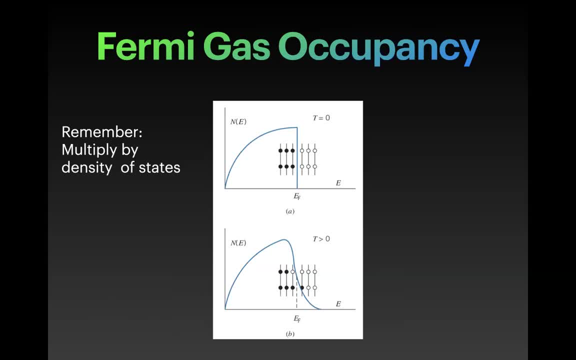 So this is a picture of you know, there's two states there because we're talking about electrons, right? So when we say that the occupancy is is one, well, you need to multiply that by the number of spin states as well. 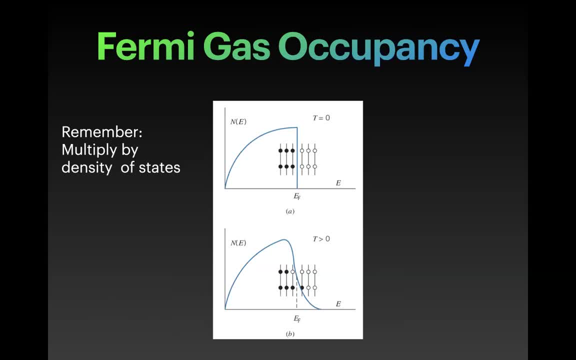 So at zero temperature or low temperature, basically again below the Fermi energy. all the states have two electrons in them and above that there's none. Yeah, so this would be like electrons in a in a metal right. We can treat the. 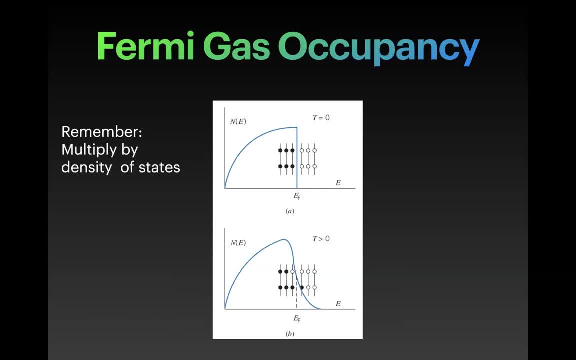 we can treat the conduction electrons in a metal as if they're a Fermi gas. But then if you increase the temperature above zero, then what happens is the Fermi energy stays the same. but what happens is basically you give some energy to some of those electrons that are below the Fermi energy and excite them above the Fermi. 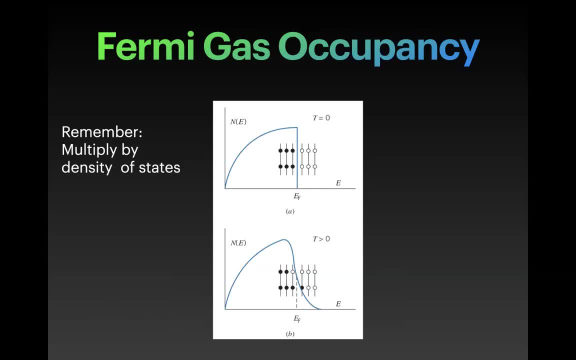 energy. So when the temperature is non-zero, then there are unoccupied states below e-Fermi and occupied states above e-Fermi, But it's more or less you know, until you get to really high temperature, you know they're mostly filled on the low end and mostly unfilled on the high end. 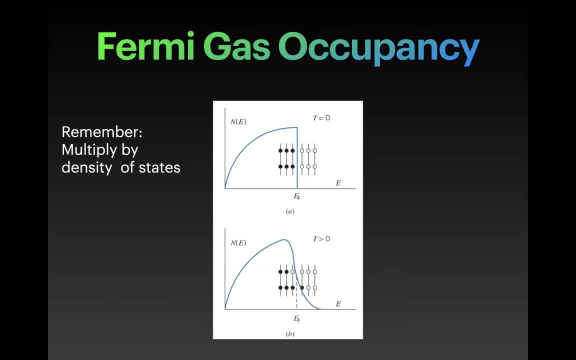 Yeah, and so this is the all the stuff that we're going to do with Fermi gases in terms of understanding, like electrons within metals, or we'll be able to use this to describe, uh, white dwarfs or neutron stars. um, all, we can treat it fairly well by treating it as. 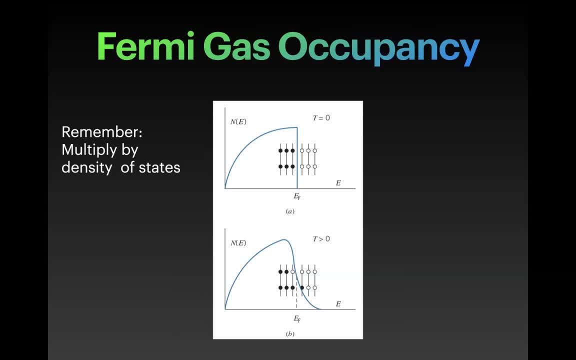 um, being at zero temperature, right, Because just as an estimate, you know, as long as you don't get well above the Fermi energy, then, um, then you can. you know these two pictures are are fairly similar, right, You've got a few that are excited above that, but if you're just trying to figure out some basic, 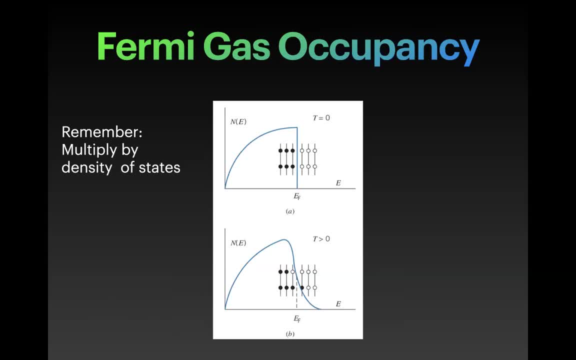 um quantities, you can treat it as if it's at at zero temperature. So this is part of the reason why I say, when I was talking about uh, neutron stars, when I say that they're at low temperature, okay, yeah, it's a million degrees, you know it's. it's low only when you compare it to the Fermi energy. 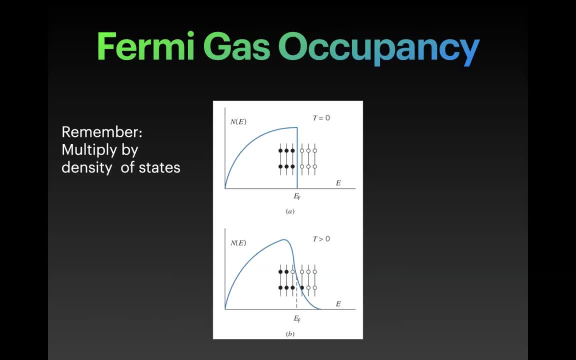 right. So the, the, uh, the temperature of a neutron star is pretty close to the Fermi energy and that's why we can treat it as a low temperature. Um, I'd have to. you know, I haven't read ahead in my. 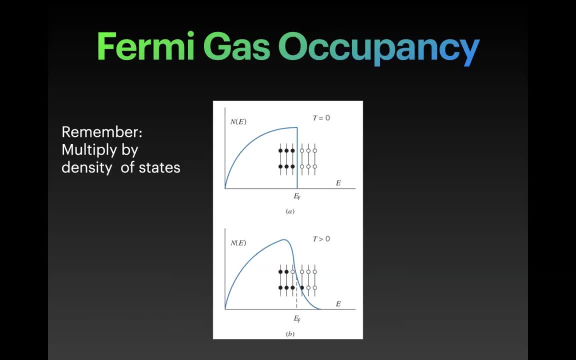 in my notes to remind myself. but I think the Fermi temperature for um for the elect- conduction electrons in a metal is something like 10,000 degrees, right, So we can treat them as low temperature at any realistic um value of the temperature. Okay, uh, and there's the uh. I forgot to. 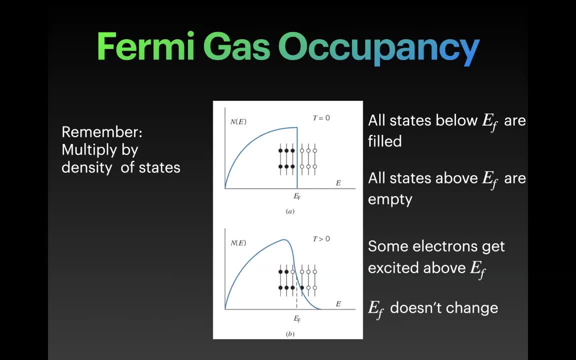 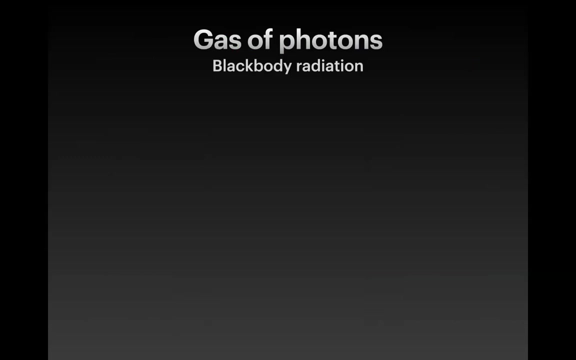 bring up the. you know, that was what I just said about, uh, the general behavior of Fermi gases. Yeah, All right. uh, any questions at this point before we do some specific uh boson gas stuff? All right, so one uh type of boson gas that we can do is a gas of photons. Um, and we skipped. 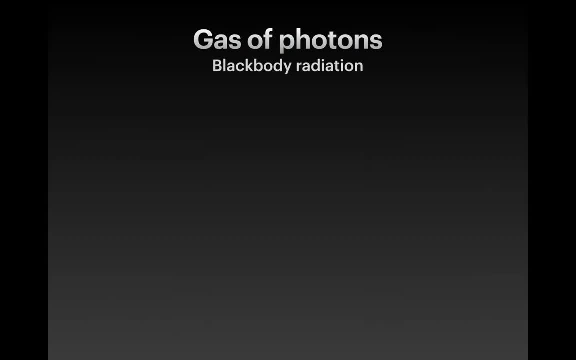 over this um, because you could l, it could beMax dollars section. in what was it? chapter three, uh, maybe about um treating light like a particle, right. so some of the earliest evidence for for quantum mechanics. so some of the earliest evidence was Planck. he came up with the idea of quantization to describe black body radiation, right, so black, 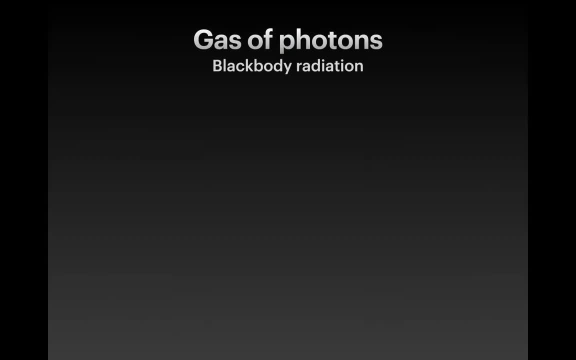 body. radiation is the electromagnetic radiation that objects give off just because they're at a certain temperature. right. so like we can describe stars this way, we can describe incandescent light bulbs this way. um the reason why, you know, heated metals start glowing red hot and then white hot. 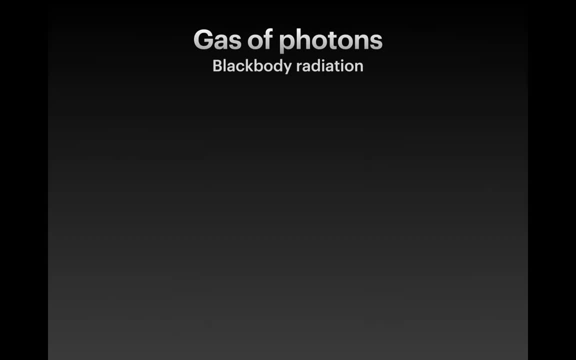 as they get hotter. um, we can even describe, you know the, the, um infrared radiation of, you know people or other, you know, just sort of ordinary objects we don't normally think of as glowing. uh, we can describe them by as black body radiation. but the classical explanations for what was going 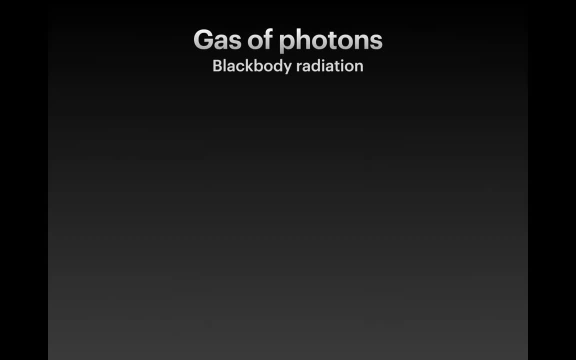 on there didn't work right. so the ideal picture of a black body is just an empty cavity with a small hole in it, and that empty cavity is going to have electromagnetic waves in it, right. you're going to have standing waves particles in a box, right. just like we've done a million times. 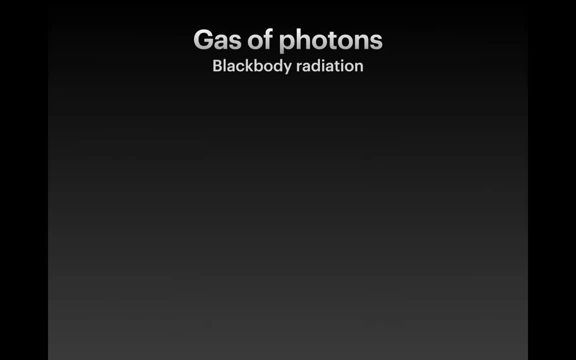 and then some of those particles will escape. but the the thing that would needed to be explained was: well, if you have standing waves, of course there's a lower limit to the wave, or sorry, there's an upper limit to the wavelength right you can only have. if i have a box this big, i can have. 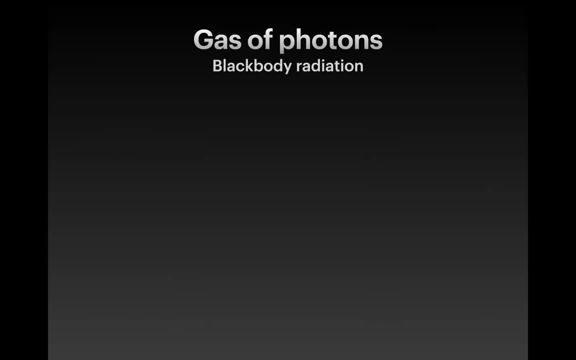 a single standing wave, right? so that's going to be, you know, like an infrared wave or a radio wave or something, depending on how big your box is, but there doesn't seem to be. you can, if you start going into ultraviolet and x-ray and stuff, right you, you can just keep putting more and more high. 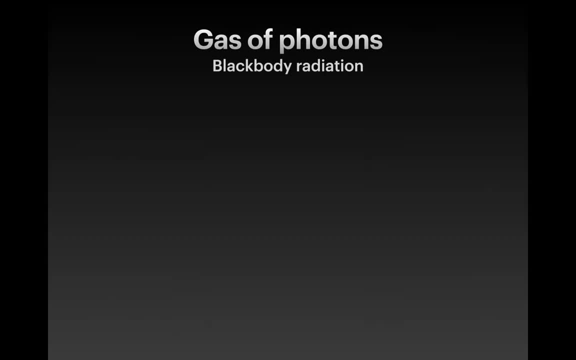 energy particles in there, because you know, once you start making that wavelength really small, i can fit anything in there. so it seemed like you know it was called the ultraviolet catastrophe, which was- it seems like there should be an infinite amount of high uh frequency, low wavelength radiation coming from a black body. but we know that's not true, right? we don't. 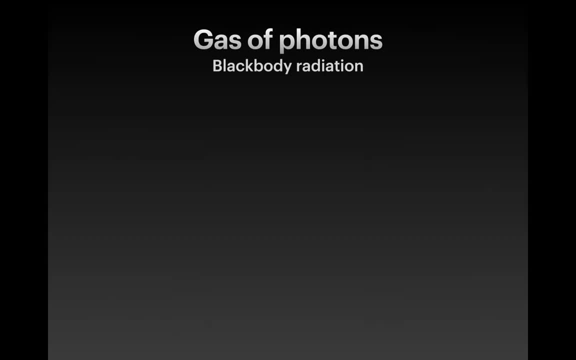 know if we can find that, but we can see. you know the shiny thing, and it looks like it's not really that. it's not the same thing, you know, as it comes to the sun, right, we get the same burst energy temperature and the blast energy temperature, and all we can do is just instantly get killed by. 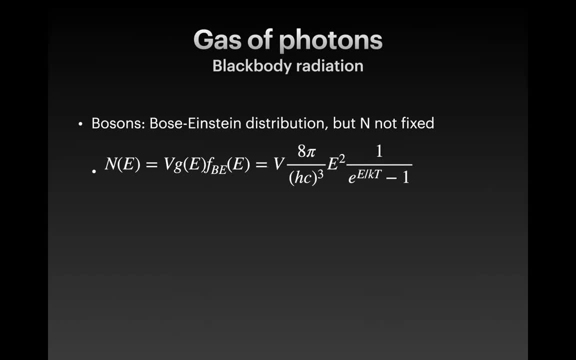 gamma rays every time we step outside from the sun. okay, so the solution is is to treat uh photons as as uh bosons. so they're going to uh, so we're trying to find, um, you know how much energy is in a certain volume of a gas of photons. 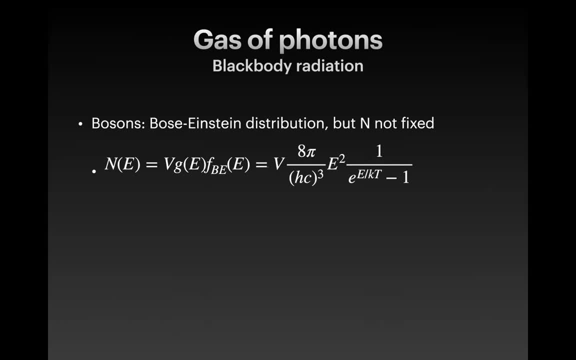 number is not fixed, right. You can always create and just destroy photons willy-nilly, right. They're constantly being absorbed and admitted by all of the atoms that would be making up this black body. So okay, so if we, if we, 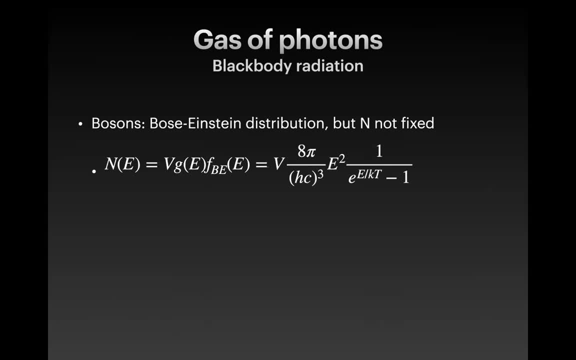 calculate the number that we would expect at a given energy right? we have our calculation here: volume times, density of states, times, in this case the Bose-Einstein distribution. Okay, so I write that out here. Recall that our density of states. here we have to use the ultra-relativistic one, right. So 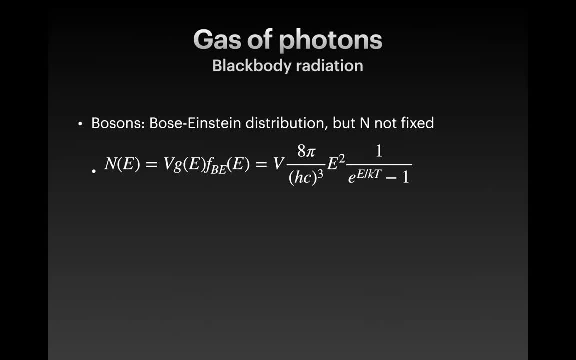 rather than going up as square root of energy, it goes up as energy squared. So I've got that factor there, And then I've got the one over exponential stuff. that is, what we just stated was the distribution function for bosons. Okay, so what we really want is the energy density right: Energy U per unit. 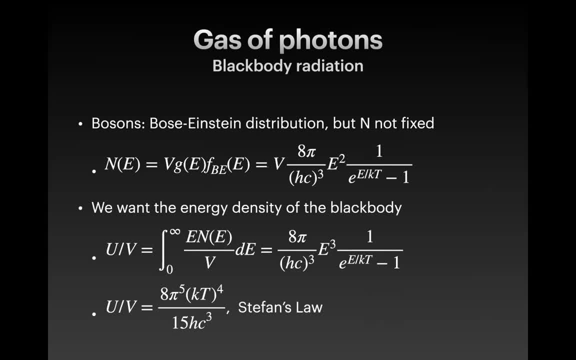 volume. So to calculate energy density, well, we would want to integrate from zero to infinity. Now we're trying to find the expectation value of the energy. So we would take energy times, the distribution function, the number distribution function and integrate it over all possible energy right. Oops I. 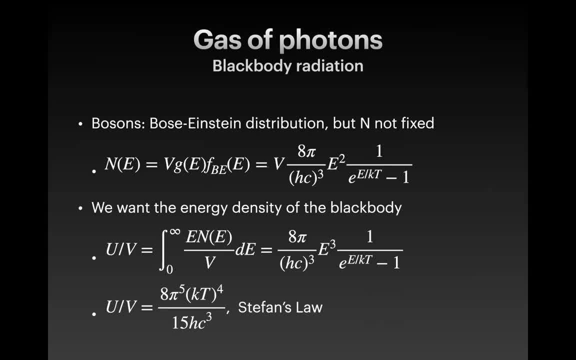 left out my integral in that last part. So this is still so okay. so I just took that first line and multiplied it by E, but I dropped the integral on accident, right? So when you integrate over that- I didn't show the steps, but if you do that, integral again. 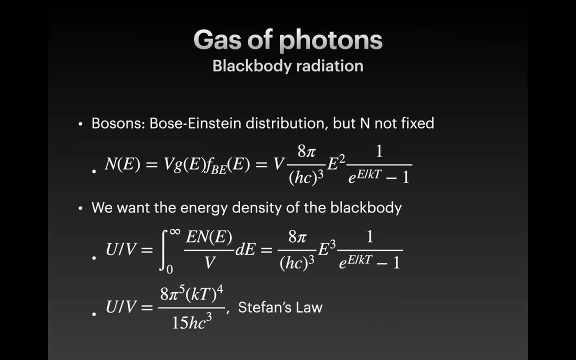 it's going to be one of these exponential integrals that you have to look up. It involves pi, always involves pi, for some reason. So it's pi to the fourth over 15.. The energy density is this, you know, numerical factor. Yeah, wow, okay, I'm. 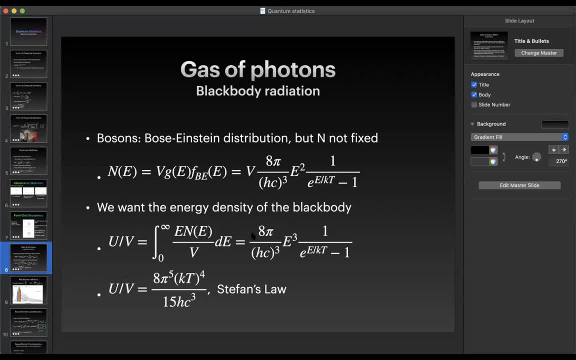 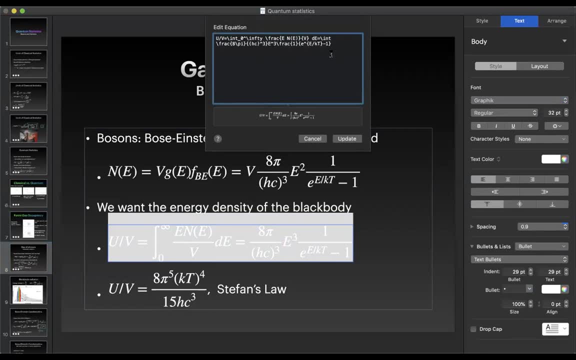 going to. I'm going to fix this because there's too many mistakes on this slide. Okay, so I'm updating that There's still the integral same limits. and then here I missed some parentheses. Yeah, that's because I made them curly braces, Okay. 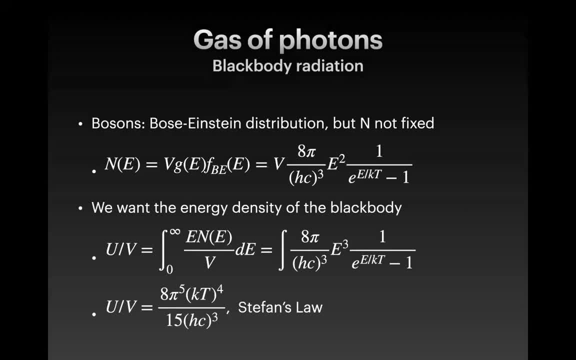 There we go. Okay, So using that I mean the important thing here other than getting the units right. but the key factor is that the energy given off by a blackbody is proportional to temperature, to the fourth power, And this was already known. 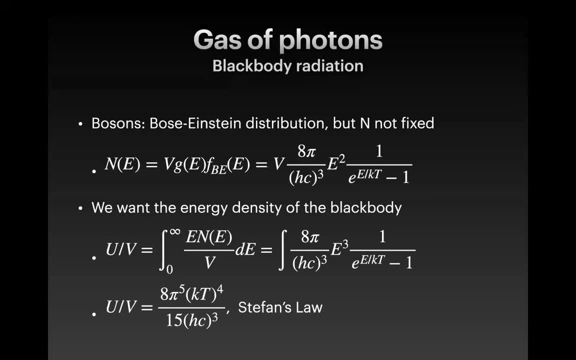 from observations. This was known as Stefan's law And, other than the dependence on Planck's constant right, they just had, you know, they just had a number that was measured, But the Stefan's law was that the energy of a blackbody 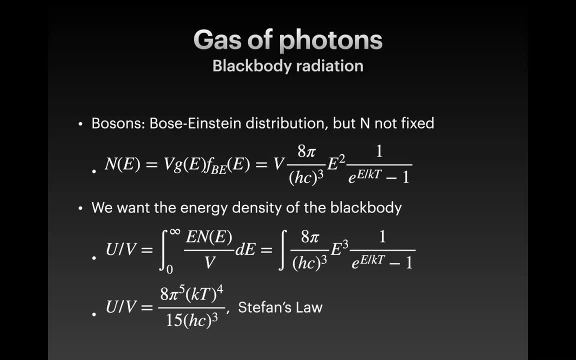 depends on temperature to the fourth power. So you can measure that you know with a given, you know temperature to the fourth power, And then you can measure heat up a piece of iron to a known temperature and then measure the energy that it radiates. 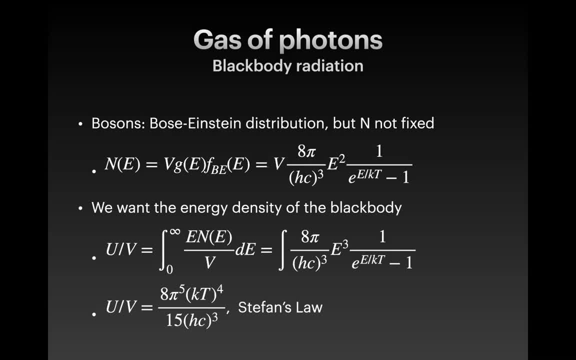 And you know, then increase the temperature and see how that changes. So this was known. So being able to find that from Bose-Einstein statistics is, you know, a good proof, or check that it works. Another thing that we can do is: 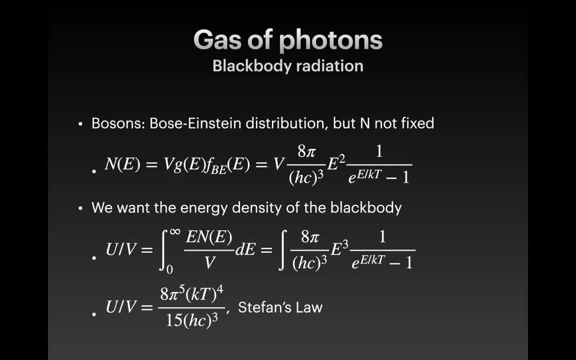 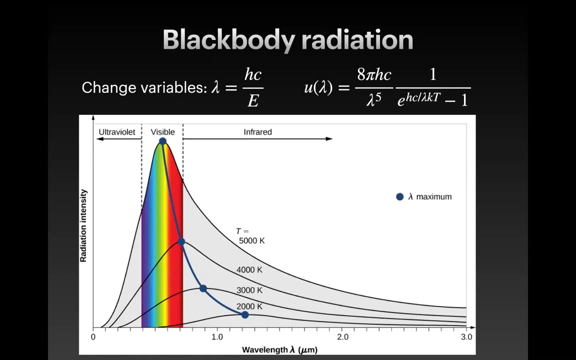 take that energy density. so before you integrate it right, so take that energy density and change it into a function of wavelength, because that's how it's usually plotted. So just with a change of variables, the familiar energy is equal to hc on lambda inverts that and then just write energy density, So lowercase u. 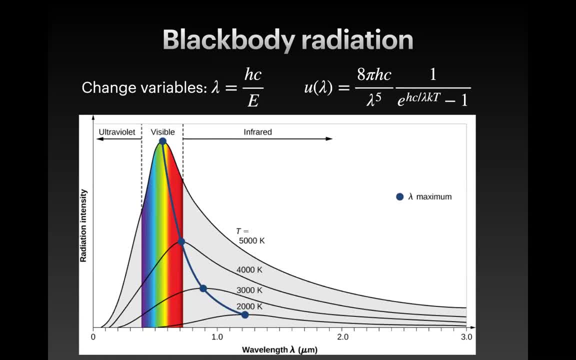 just means energy per unit volume. Then we get this expression, and this is how, how these things are usually plotted. So this is the intensity: radiation intensity plotted as a function of wavelength for several different well, it doesn't matter what they are, whatever black bodies you have. So it could be a metal. 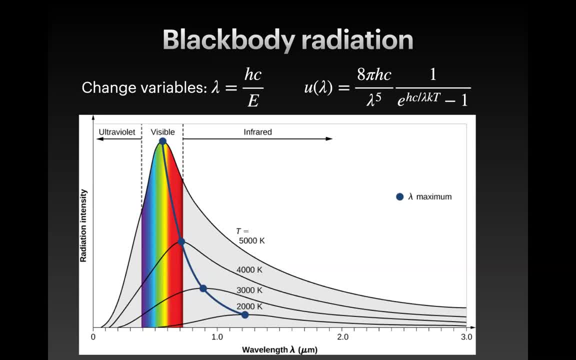 or it could be a star, which is where this is often applied. So plotting that at different values of the temperature, you can see they're labeled there. You can see, not only does more temperature mean more total energy is going to be given off. 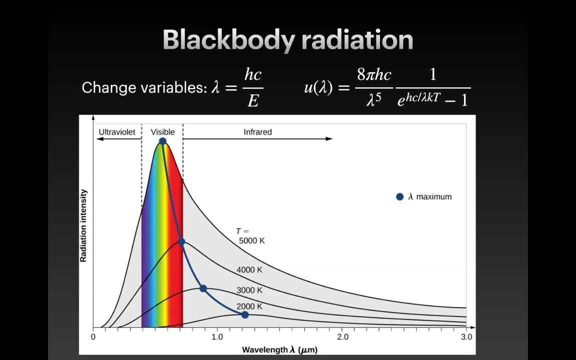 right, it would be the area under the curve. but it also changes where that, at what wavelength. that peak, that energy peaks right. So at 2000 kelvin, pretty hot right, 1700 celsius, which is, I don't know hot in fahrenheit. 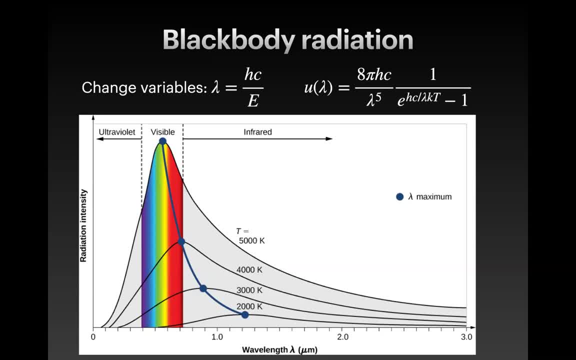 The peak is still going to be in the infrared or the far infrared right. it's not that close to the visible spectrum, but you start to get some visible light given off. So at that point, probably between two and three thousand kelvin, you would start to say something is. 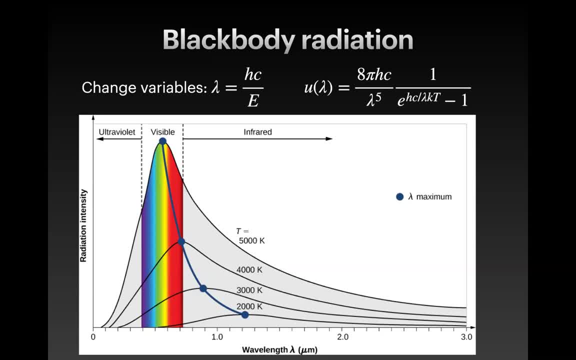 glowing red, hot right, because even though it's peaking still in the infrared, it's going to be giving off a lot of red light, So it's going to, but not that much blue light, and so it's going to look red. 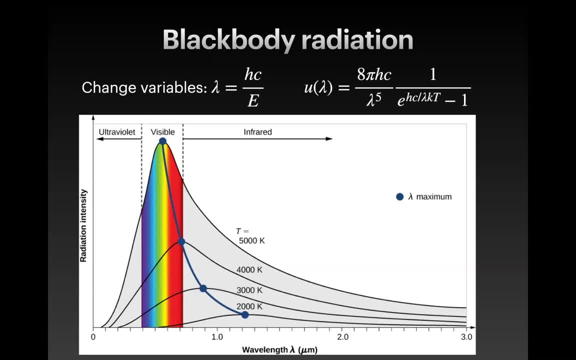 And then you know, as you start to get to 4000 kelvin, now you're seeing a lot of visible light being given off. Of course there's still a lot of infrared light, which we feel is heat, or infrared radiation, which we feel is heat, being given off. so you're going to feel that as well. 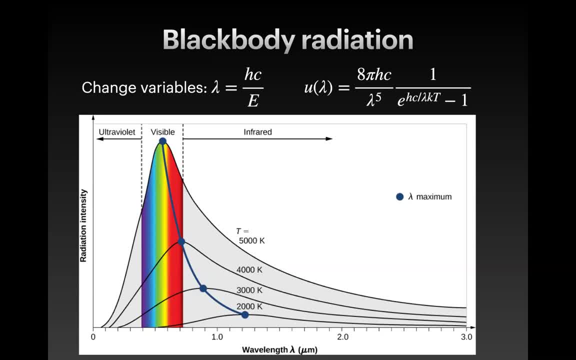 But it would start to have much more broad spectrum, and so we would say things start to glow- white, hot, Right, and then peaking in the middle of the visible spectrum, green to yellow, that's. I mean. sunlight peaks in the in the middle of the visible spectrum. so does incandescent light. Now 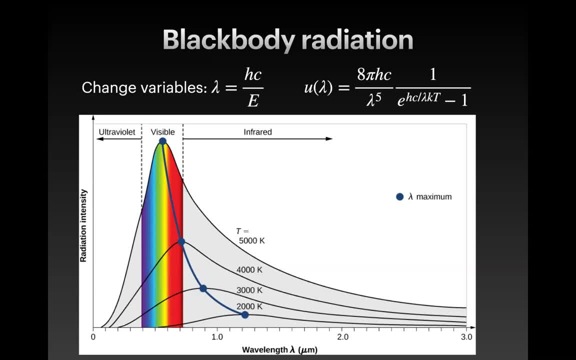 that's not a coincidence, probably. We probably evolved eyes that allow us to see the in the part of the spectrum that the sun gives off most of its light. So you know, that's why a tennis ball, you know you're going to see a lot of light in the middle of the visible spectrum. 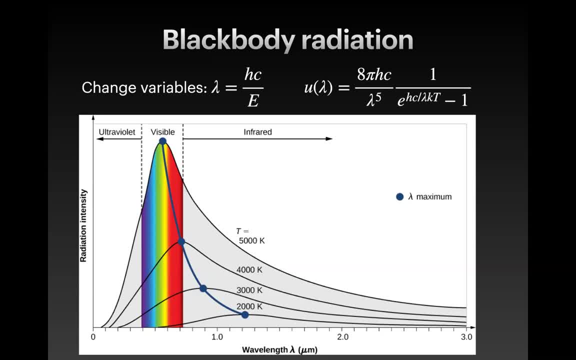 So you know, a lot of what is visible is also visible, but you can see that, like I said right now or when I turned it on, that you could see things that are red, right, like you know, a little bit of yellow, but you really don't see things that are red. 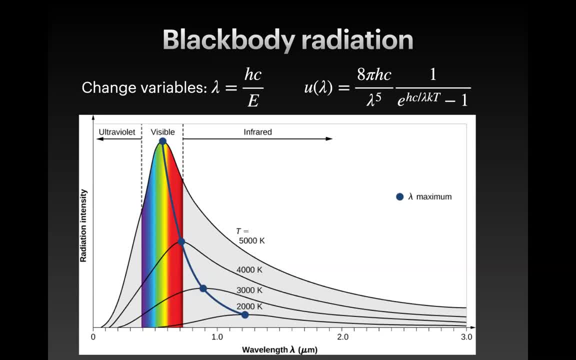 So you know we were seeing, you know light, a little bit of yellow, and we're seeing. or if, if you're a student, you see light that is red, but if it's not, you know, if it's not real light, right then it's still uh, it's still gonna be the light that's visible. 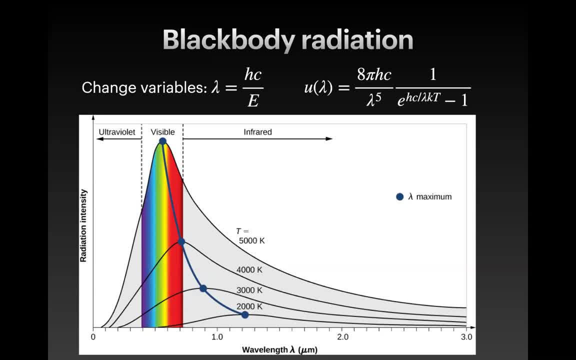 So it's not that that's the only thing that we can see, But I mean, we still have internet. but I do think we're seeing a lot of light. tennis balls are dyed right. They're not glowing 5,000 Kelvin, So if you just took that expression, 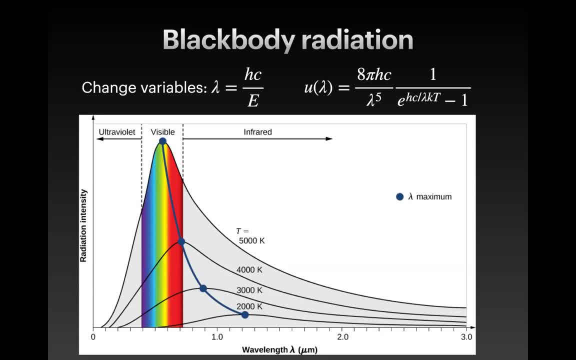 as a function of lambda and you took its derivative set, that equal to zero, solved for that. you would find the peak wavelength as a function of temperature and you'd be able to reproduce that plot. And that was also known before quantum mechanics. It's called 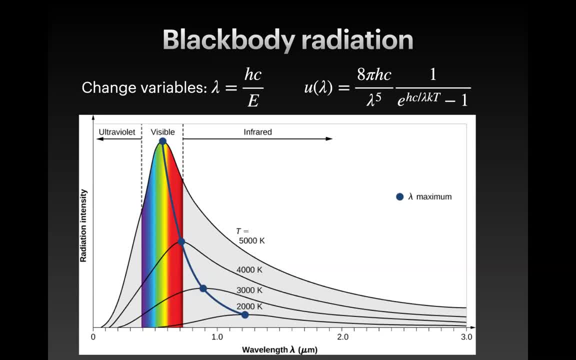 Wien's displacement law W-I-E-N Wien, And so that was another confirmation of this. you know this math, that it was able to reproduce what was already observed, but explain it for the first time, And so the explanation of blackbody radiation, along with 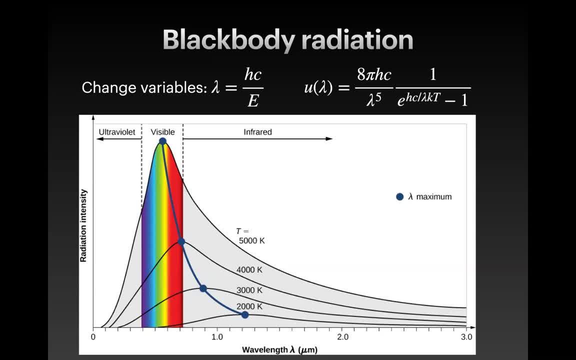 the photoelectric effect were really the things that proved the usefulness and correctness of quantum mechanics. All right, so we're going to wrap up here. We're going to move on to questions. before we move on, All right, I hear my dog telling me that the mailman is here. Hopefully she can handle it. 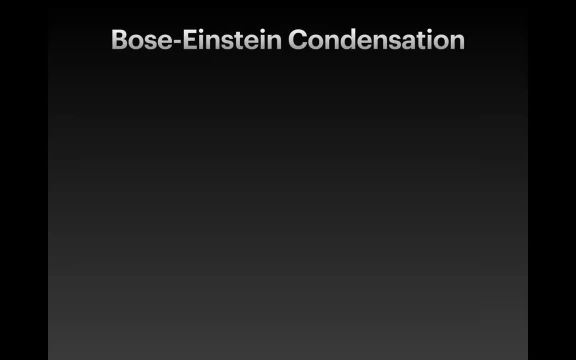 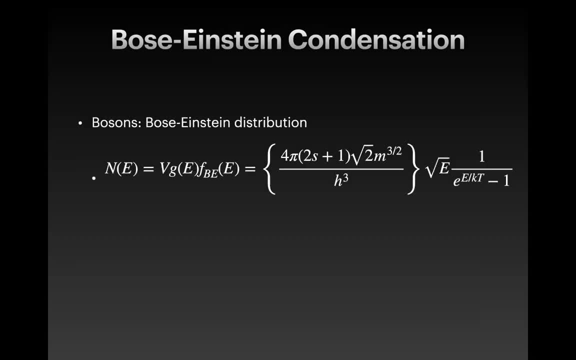 And then I'm going to give you a little bit of time to think about this, Based on his topic. So let's look at. so this here we're going to go to, to bosons that are non-relativistic, Right, so not photons, So they can't be created just out of thin air. 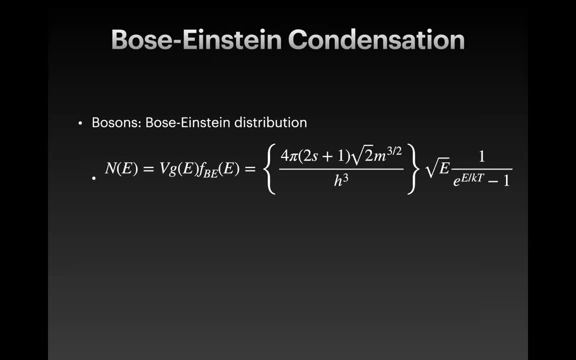 And they have a different density of states. Right, It's the one that goes as the square root of energy, and not e squared, And then you've got that whole, whole mess of stuff in brackets. So this is what you know. we came up with this on Friday and we're 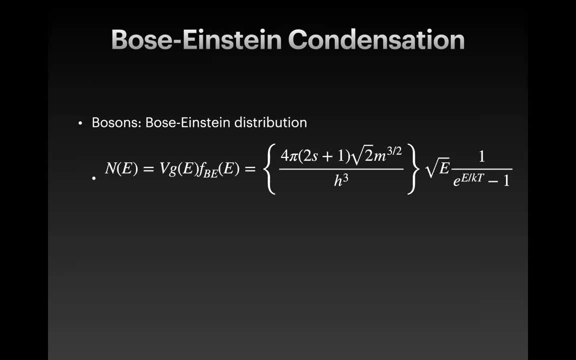 going to use it now. So now again, I've dropped that normalization for that A for the bosons, And the reason for this case is that we're looking for- we're going to try and look for- the maximum number of bosons that can fit in a particular volume, right? So when we calculate this, 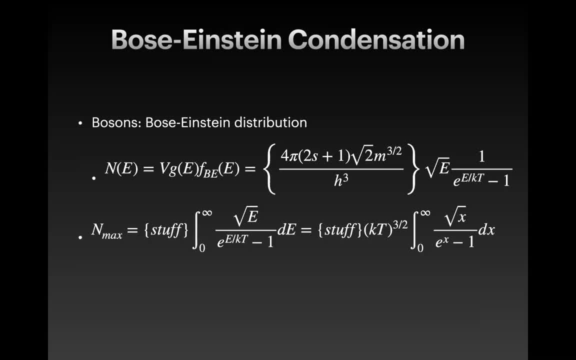 integral. we're trying to find the maximum value. So if you had something other than one down there right, If you had a factor of two, for instance, well then you'd get. you'd be dividing by something in the denominator and therefore you get a smaller number. 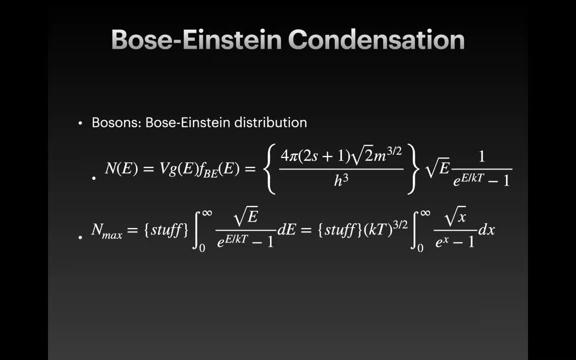 right And it can't be anything negative, because that would mean- or anything negative would mean- that you get a smaller number. So if you had a factor of two, you'd get a smaller number. So if you had a factor of two, you'd get a smaller number. So if you had a 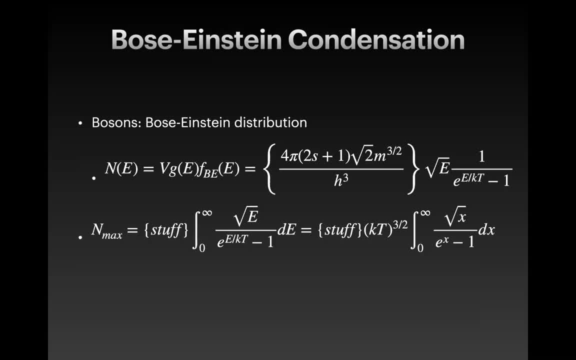 anything smaller than one, because then that would allow the denominator to sometimes become negative, and you can't have a negative distribution function. It just makes no sense, right? You can't have a negative probability, Okay, So to get the maximum number. 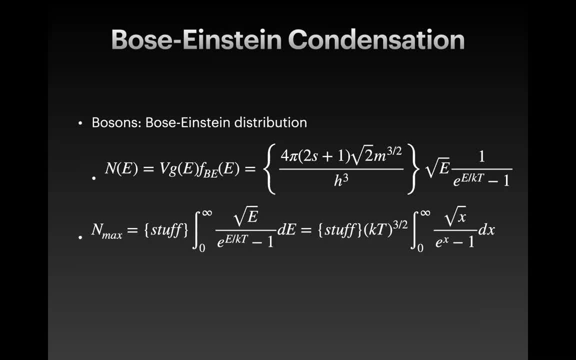 we let that normalization be one, and that also makes our life easy. Okay, So we want to calculate N. So we're going to integrate from overall energies. So we've got stuff right, That stuff in braces, The integral from zero to infinity, of this square root of E. 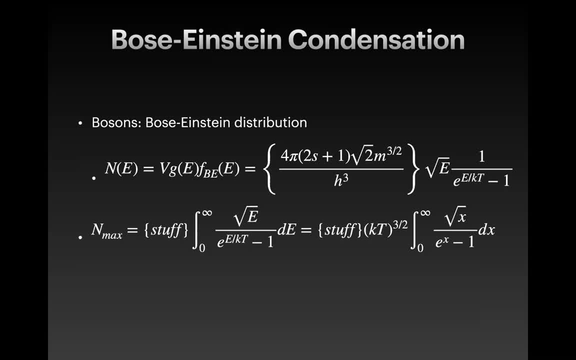 divided by this exponential minus one. So again, just as a reminder of the general technique, of what you need to do for these type of integrals, we would do a change of variables, And here I called it X just because we already used U for energy density, So I didn't want to get that. 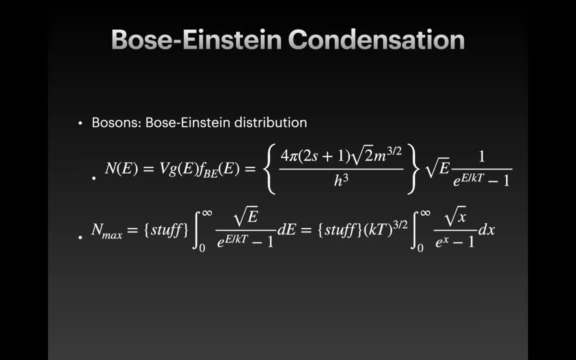 confused, but you can call your variable whatever you want. So we would just use again, as we have been, E over KT is our X, And so we're going to get this dimension full factor out in front of KT to the three halves, And then we've got that integral and 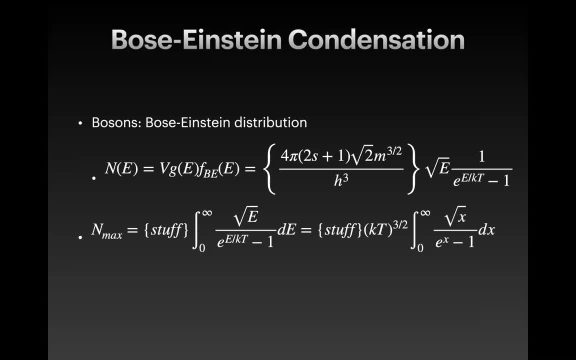 it's going to be some number on the order of one and we may or may not be able to figure it out. So anybody have any guesses Wrong? Okay, It's okay, there's a square root of pi involved, You know. you probably guessed it if you had. 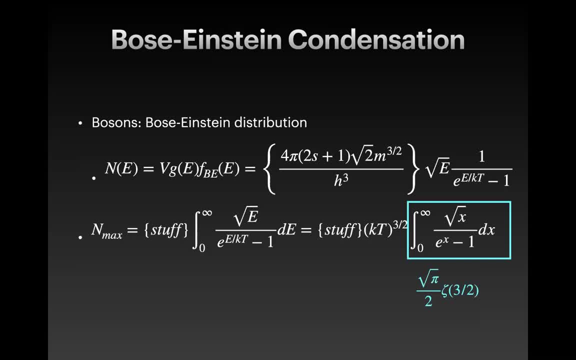 guessed anything that there would be a pi somewhere. And then there is this thing, zeta of three halves, That's known as the Riemann zeta function And it's got some weird properties if it's related to the number, to the prime numbers, And I think there's a millennium prize related to. 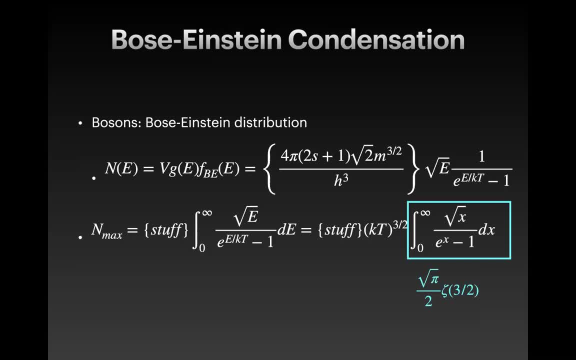 like figuring out some properties of the Riemann zeta function that you can win a million dollars for solving. But we know how to calculate it, or somebody does. It's not a nice looking number, So too bad. You can keep it in there or you can just. 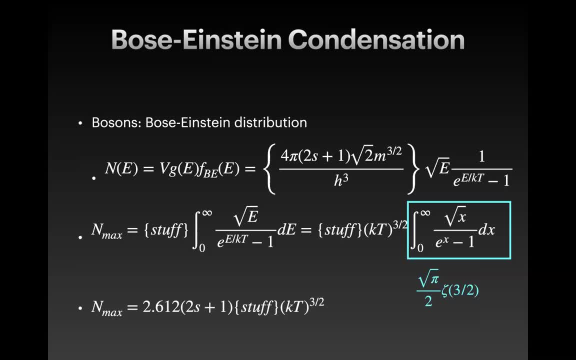 put things in decimals, So we get this gross looking thing. Okay, that 2.612, it's actually dot, dot, dot, dot, dot, right, It's not going to be an exact value. And then we've still got oh, 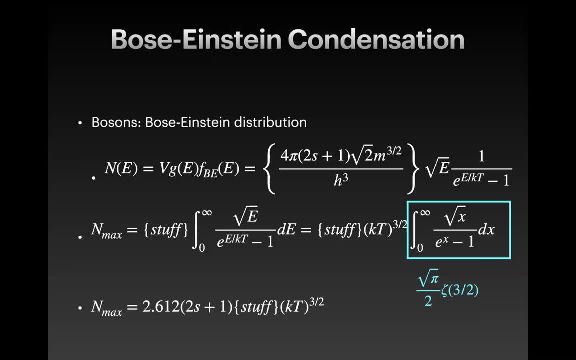 I don't. I accidentally factored out the the spin part from the rest of the stuff So you could stick it back in stuff if you wanted And then times KT to the three halves, right? So you've got number times, dimension, full stuff in. 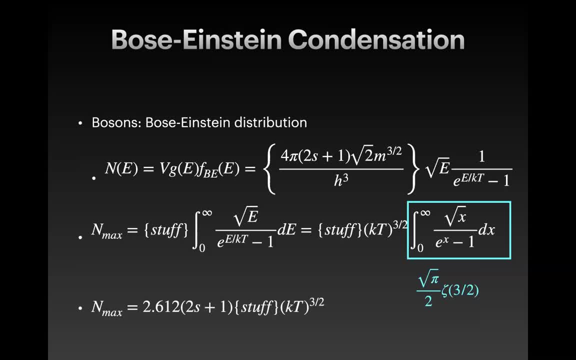 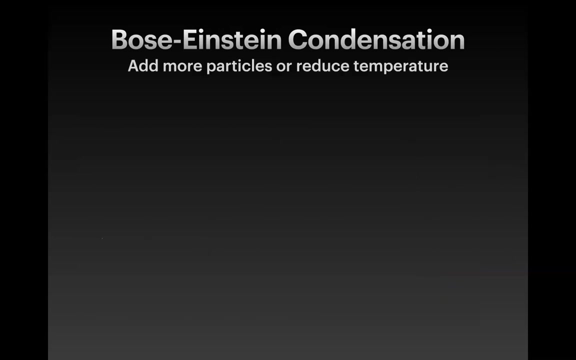 braces, And then times KT to the three halves. That's going to be the maximum value of bosons that it seems that we can put into a container. Okay, Great. What happens, though, if we try and add more particles Or if we have a gas? 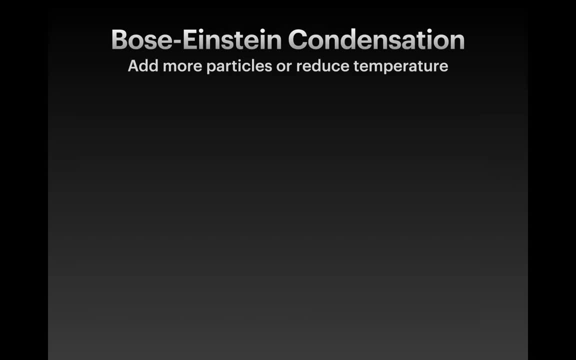 that has the maximum possible number for a given temperature and we reduce the temperature. Where would they go? Well, let's take a closer look at the energy equals zero state. So our math is telling us: okay. so we've got our distribution function for bosons as energy goes. 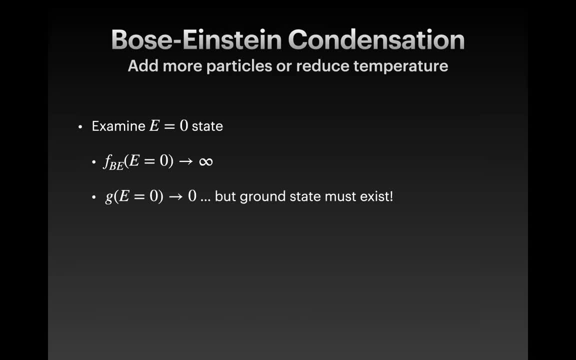 to zero. That goes to infinity, But that's okay, because our density of states, as energy goes to zero, goes to zero. So when you're multiplying those two times each other and you integrate it, your integral from blowing up. however, we know that any quantum system has to have a ground state. 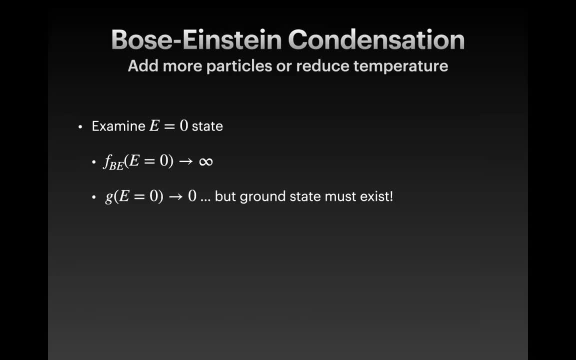 right, there has to be a lowest state that has particles in it, because we can kind of prove this by contradiction, right? if you said, um, well, there's- uh, there's emptiness, and then there's the first filled state, then you would just say, well, if there's emptiness and nothing's allowed. 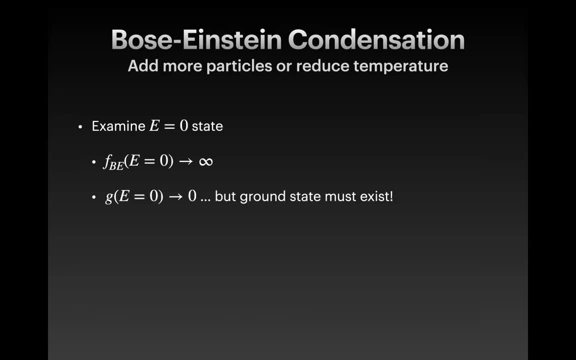 there, then it's not, then it's, you know, not physically true, not physically meaningful. so the first filled state is the ground state, and we just rename that. you know you would measure all your energies from the ground state, right? so the ground state must exist and it can't be empty. 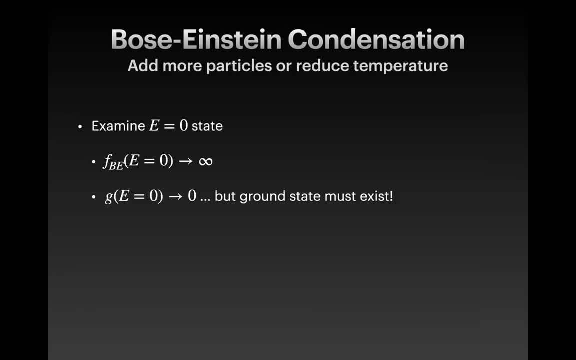 so even though our math says that, you know that from the density of states it goes towards zero, there must be a ground state so it's not actually empty. there could be one particle there. but if there can be one particle there and they're bosons, then you can put another particle there too. right? fermions are not allowed. 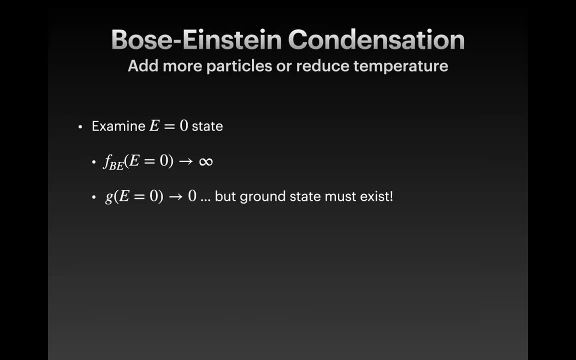 they don't like each other, right? they? fermions are social distancing bosons are on spring break, um, so you know that that's basically um. what happens is the. the ground state becomes the florida beach is of uh, spring break, um, and you can just start putting particles in there. 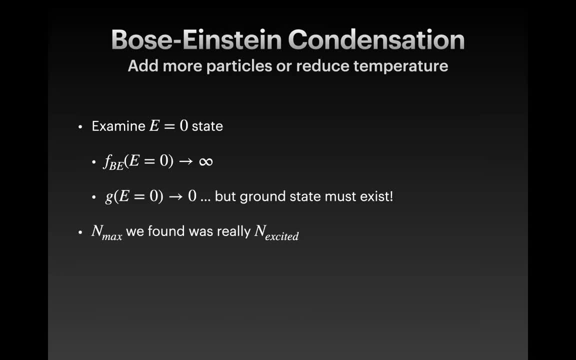 uh, technical term, you can put particles in there willy-nilly, so um, this maximum number that we found was actually not the maximum number. it was the number that were in excited states, right, so it's the number of particles that are not in the ground state. that was what we actually calculated. even though we called it n max, we were diluted. 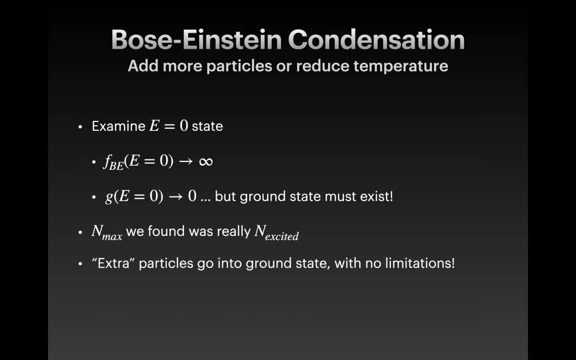 so the extra particles go into the ground state with no limitations. so the total number of particles then is going to be equal to n naught, the number of particles in the ground state plus the number in the excited state, which is what we had calculated. okay, so where does this start happening? because above a certain temperature, 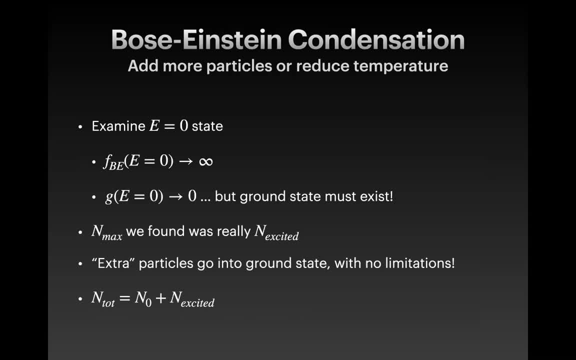 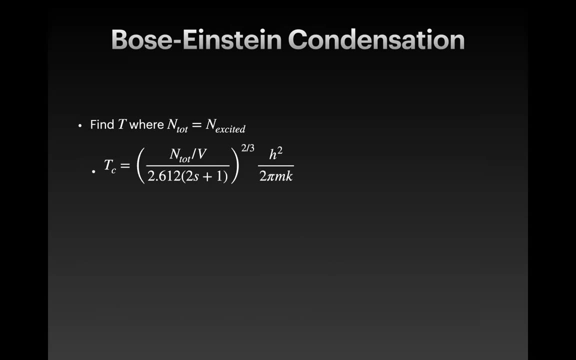 right, there's basically no particles in the ground state. i mean there might be one, uh, there has to be at least one, but there's, you know, as a percentage of you know, you got moles worth of particles and one is in the ground state. it's basically zero. so if we find, uh, the the temperature. 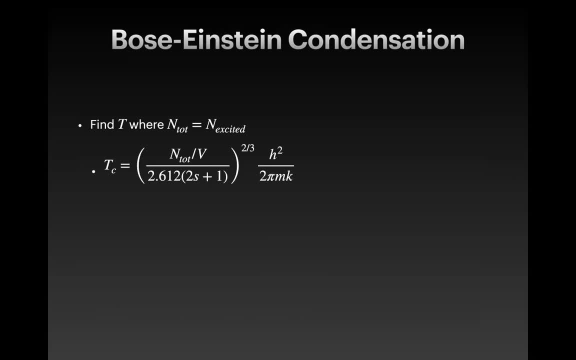 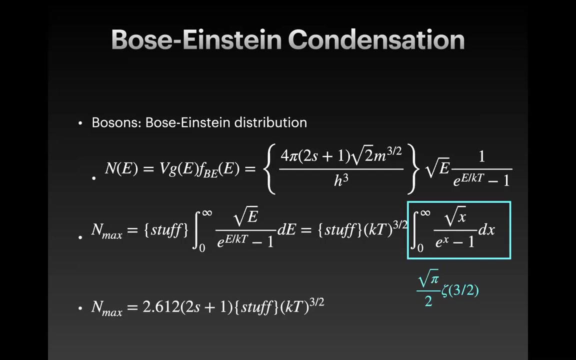 where n excited is equal to n total- basically no particles in the ground state- you can calculate what's called a critical temperature. so you basically take um, go back, not that far, and you take one of these four. you take this uh expression at the bottom with stuff you know written out, and solve it for. 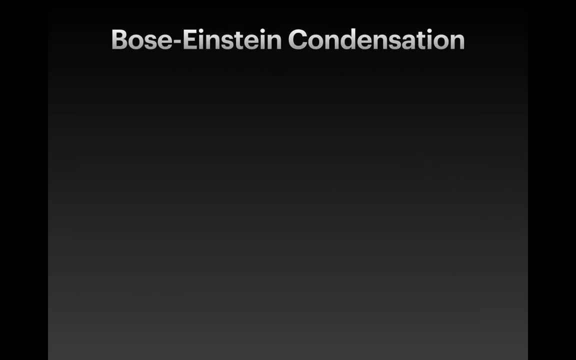 temperature, right, and uh, invert that and solve it for temperature, and so when you do that, you get the critical temperature where you have filled all the possible excited states and that's calculated here. um, it's going to depend on the, it's going to depend on the volume which makes. 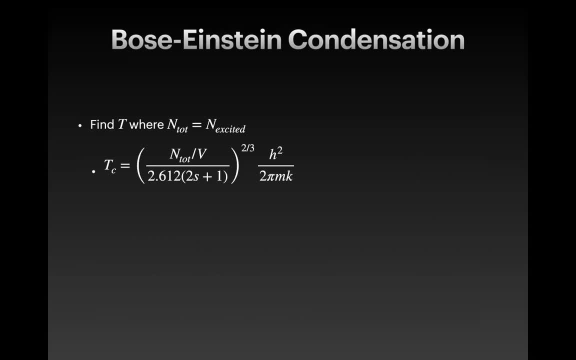 sense It's also going to depend on the, the mass of the particle right. so a more massive particle is going to have a lower temperature where this starts to occur. And then you can also find so by taking that n total and subtracting the. 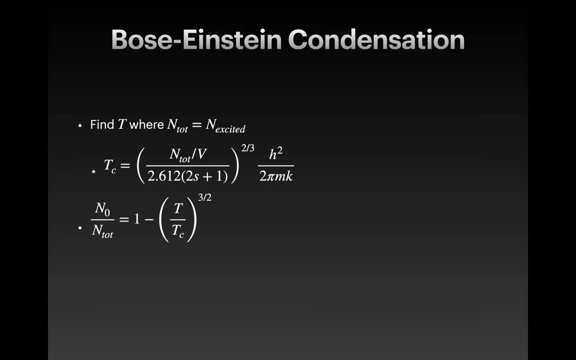 n in the excited state and solving, you can find this nice concise expression which is the fraction of particles that are in the ground state Right. so basically, at when the temperature is equal to that critical temperature, there are no particles in the ground state. they're all in excited states. But once 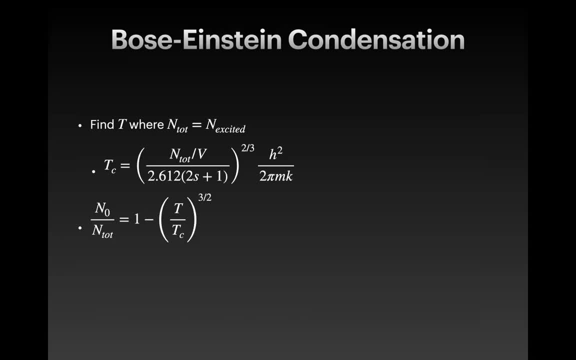 you if you're reducing the temperature rather than shoving more particles into your container. if you reduce the temperature, then you're going to get more and more particles into the ground state into the ground state as you reduce the temperature. So all the particles are in the ground state. 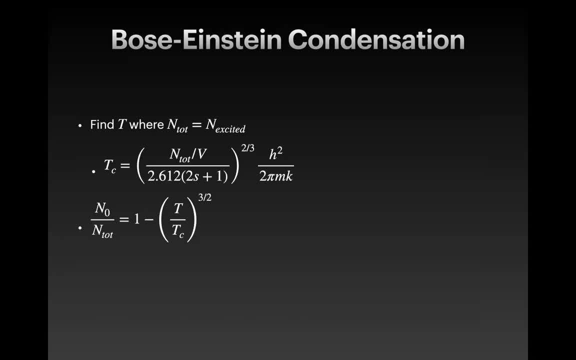 they're all all in the same quantum state. so, uh, weird stuff starts happening. um, yeah, so for an ordinary gas, um, if we take the density of an ordinary gas, it's uh like 10 to the 25th per cubic meter. so if we calculated the critical temperature for that, um, it would be about one millikelvin, which is 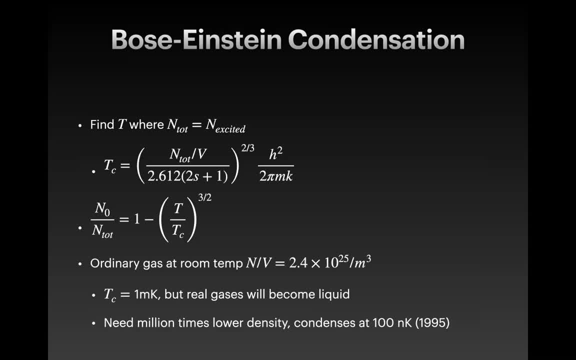 cold enough, uh, but a real gas, right. so if you said: well, let's do this. what's a boson? uh, oxygen is a boson. helium four is a boson, right. anything with an integral spin, uh, in the nucleus, uh is a boson, um. so you know, helium four is a good example. well, you would actually create liquid helium if 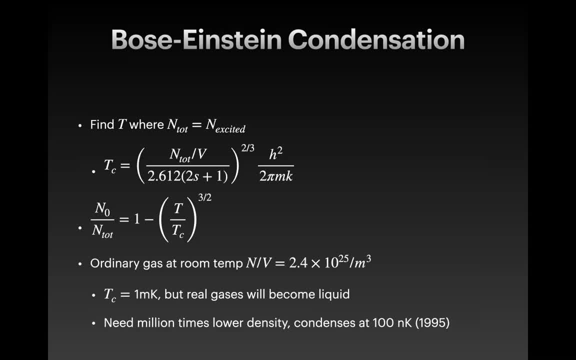 you just kept the density. you know, if you took a tank of helium like from a even just a balloon shop, right, that's someone's gas and you know you can't get the density of that gas to the nuclear system, right? so if you take that helium tank from the balloon shop and and cool it down to one, 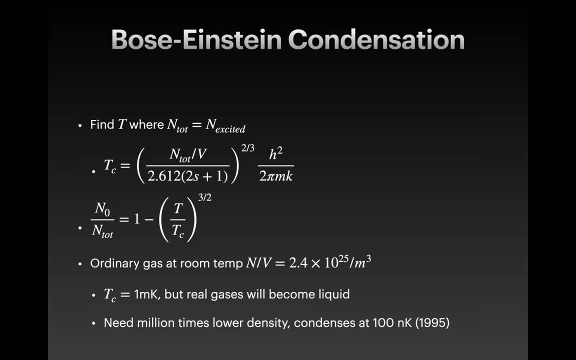 millikelvin. it's going to become a liquid before it would ever get into this Bose-Einstein condensate, right? so this is not a condensation in the sense of something becoming a liquid. it stays as a gas. it's just that a lot of those particles then jump into the ground state. so you need a the 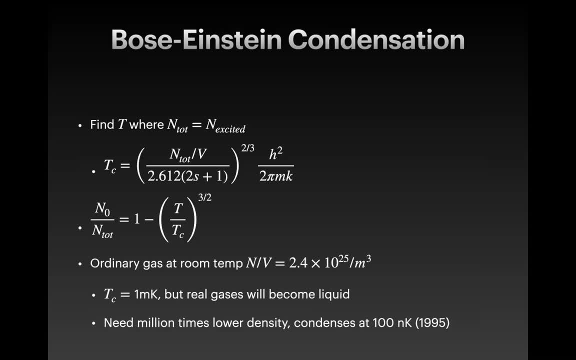 density from a practical point of view, just because real gases do become liquids- um, about a million times lower uh density for something like helium-4 uh and it condenses at about 100 nanokelvin. so really really cold um, and that that was first achieved, i actually remember. 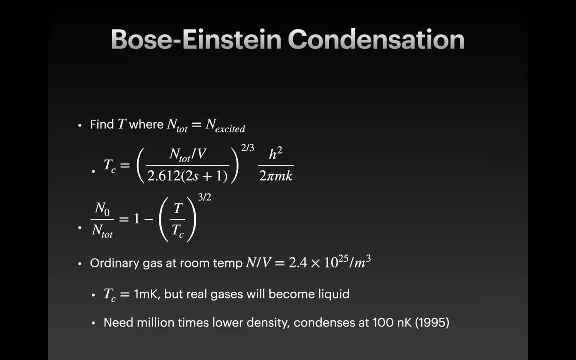 reading about this because i was a nerd. um was a nerd. um, as if i'm not still- in 1995, um, my family had a subscription to scientific american, so i remember reading about this. um. so, using a combination of laser cooling and magnetic cooling, after doing the normal sort of refrigeration and uh diffusion techniques, um 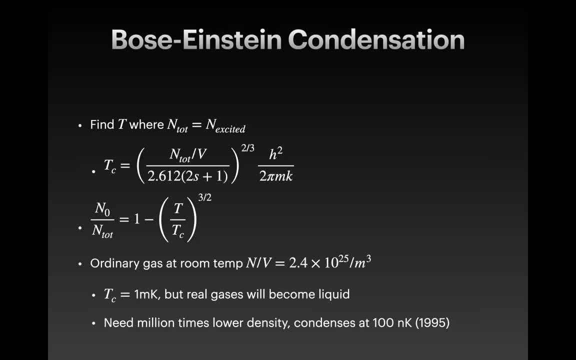 this was first achieved. and then you know pretty quickly, uh, that was awarded a nobel prize. so you know it's named after einstein, right, einstein was not alive in 1995.. uh, so the you know this, uh, and bose- i mean well, i don't know when, when bose died, um, probably was not alive either. 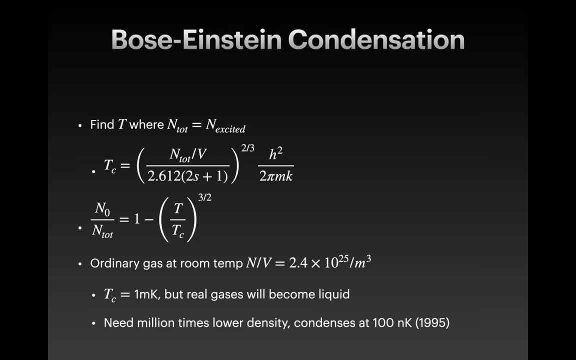 but you know this was 1920s, 30s, that this was first predicted and not experimentally observed until until the mid 90s, um. so you know, uh, on, i didn't, you know, we, we wouldn't have time to really get to it anyway, but so i didn't prepare um sort of like the examples. 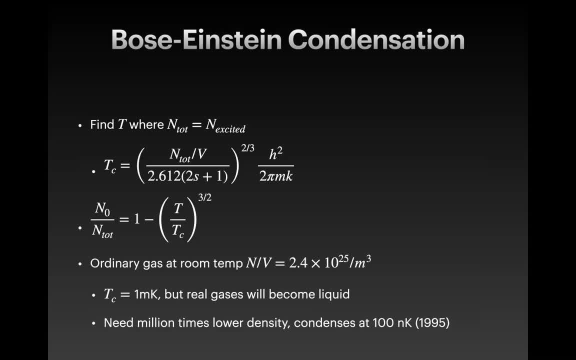 but what really happens at this low temperature is that all these particles, they go into a single quantum state, so they really act as if they're a single. they're a single quantum system and so weird, um weird things start to happen, uh, because of that. so we'll go into that, uh, in more detail. on, 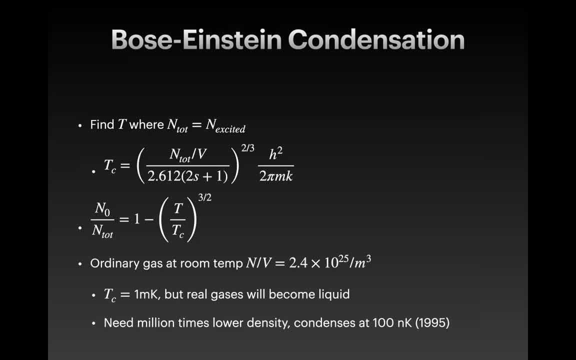 on wednesday and also do some of these, uh, fermi gas examples. so that's, uh, that's what i had for today. um, any questions at this point? so i just have one question where you said to the beginning, you said: fine, t or n, total equals, and excited. 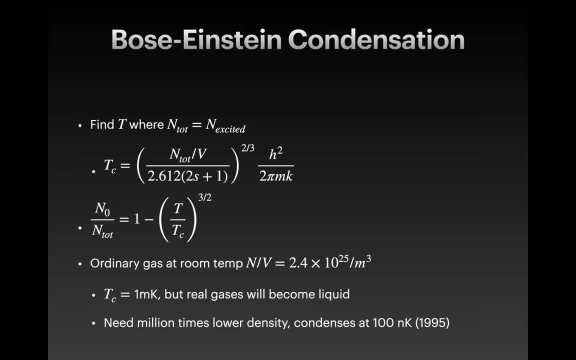 but in the previous it's like: is that the ground statement? it must exist, right so? uh, make one of those lines and the equal sign squiggly, i guess. right so there'd be like one in the ground state: uh, at temperatures above the the critical temperature. 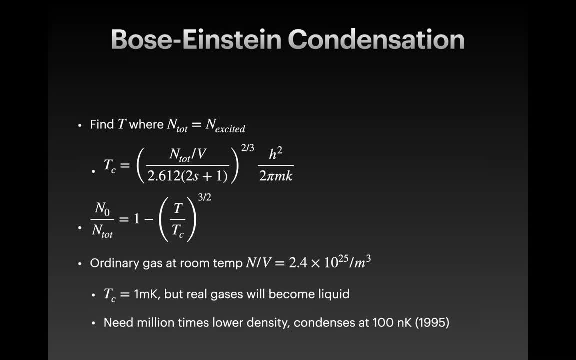 but that's basically zero when you're talking about a gas of of molecules. so, yeah, cool, because if you think about, uh, you know, zero energy or the lowest possible energy, that would mean no kinetic energy. there really is only one way to have no kinetic energy, and that's to not move at all.